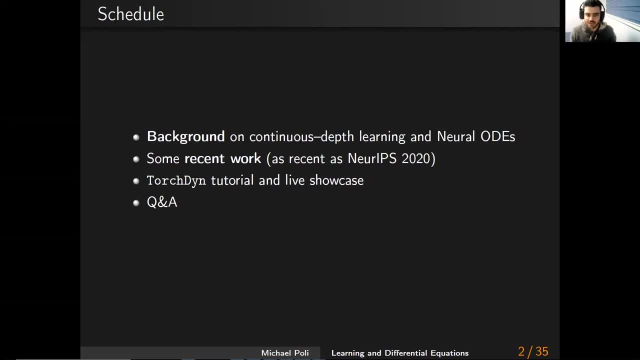 I will give you a little bit of background on what continuous depth learning means, what the objectives are and why we should care as a community. A lot of this content will be relying on will be focused on neural ordinary differential equations, which are not everything. 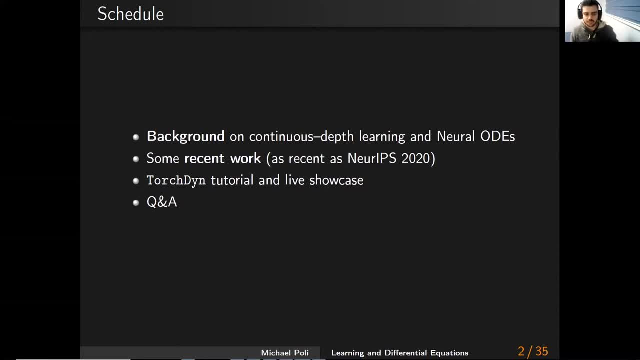 they're a core component of the field and they're a good instructive first step into the field, since it's a very clean, very simple way to say, a way without too many assumptions, to merge differential equations. So, in particular, it's important to focus on the fundamental structure of the neural networks. 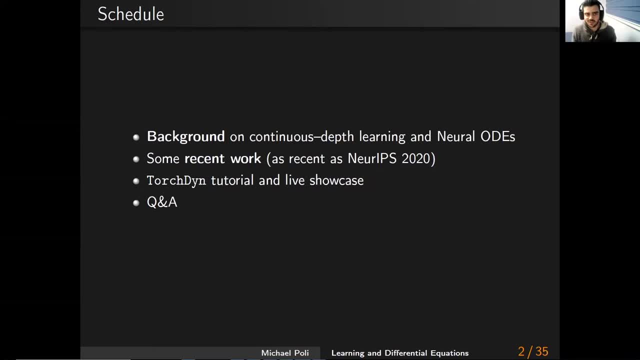 and neural networks In particular, merging a very specific type of differential equation, which is arguably the simplest one, the most well-behaved ones: the ordinary differential equation. We'll then take a look at some of the more recent works, including some of our papers going beyond ODE's. 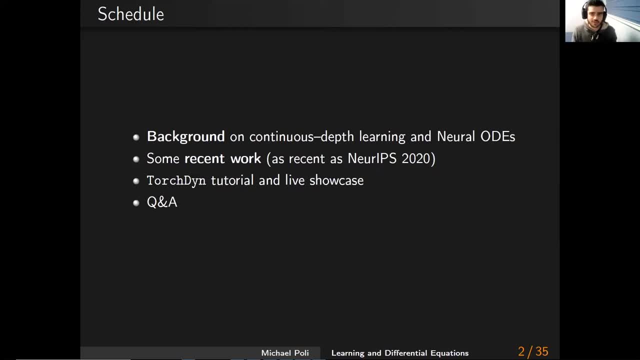 maybe to other classes of differential equations. All this would be taking around 35 to 40 minutes, And then we'll look at a library that I co-developed with some collaborators, all dedicated to neural differential equations and continuous step learning. We'll show you what is possible in around 10 minutes. 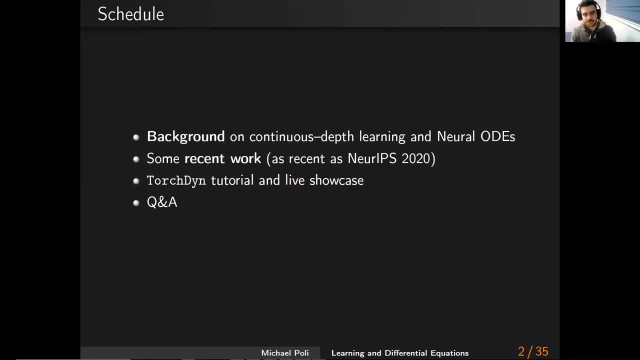 and how you can change some of the templates for your own applications, And then we'll finish with the Q&A. So I'd like to say that you won't see, aside from the live code walkthrough, you won't see as many discussions of results and applications. 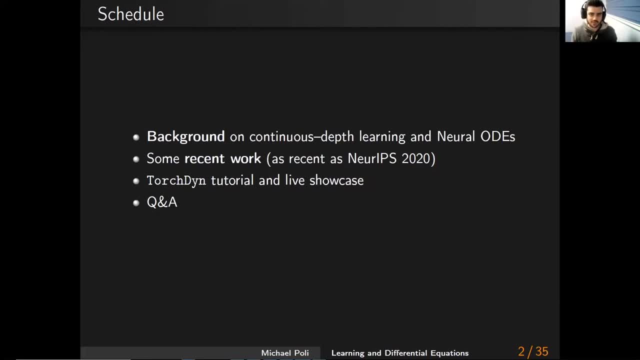 I'm trying to give you as broad an overview as possible, with enough technical content that, with the help of nine tutorials, as well as one or two references, you'll be able to then go on your own and really focus on the specific applications that you care about. 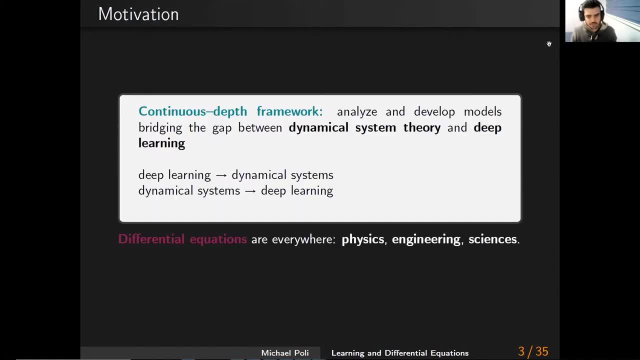 be it finance control or whatever you Okay. so continuous step framework. We are somewhere around the intersection between many fields: deep learning, machine learning, dynamical systems and thus differential equations. What is the? what is the object, the final objective? 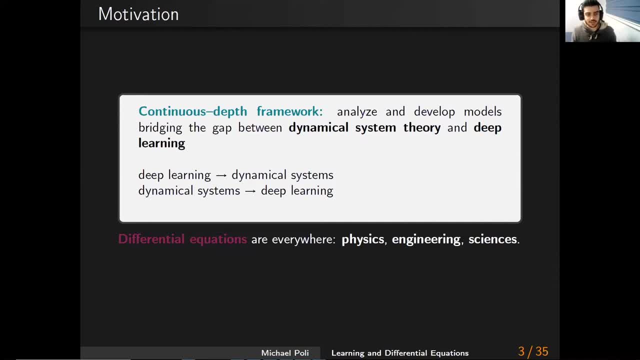 We'd like to have the same type of types of successes that we've had in other traditional machine learning fields, such as computer vision and natural language processing, but that haven't had the same type of widespread use yet. So something like physics, the broader sciences, 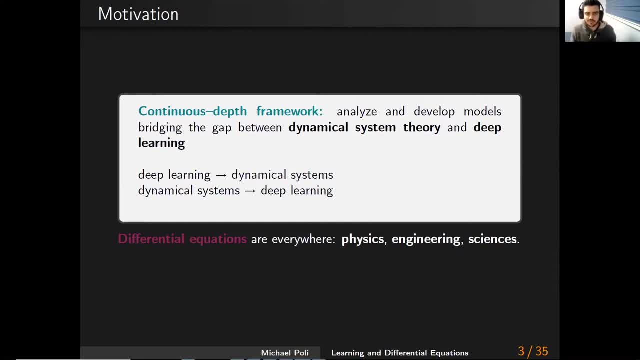 medicine finance. that have been where some of the other methods, classical methods, have been applied, but they haven't yet reached mainstream usage or deployment. To do this, we need to go beyond what we what we know deep learning models to be. 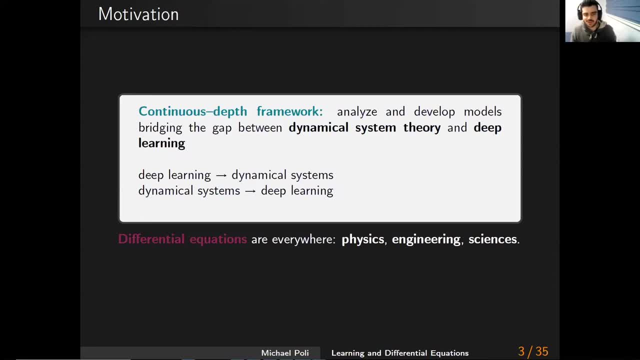 And some of the people in this field often refer to this symbiotic relationship between deep learning and dynamical systems. Indeed, some people are working on one direction. They're working on injecting more deep learning and machine learning into methods to help dynamical system research, differential equation research. 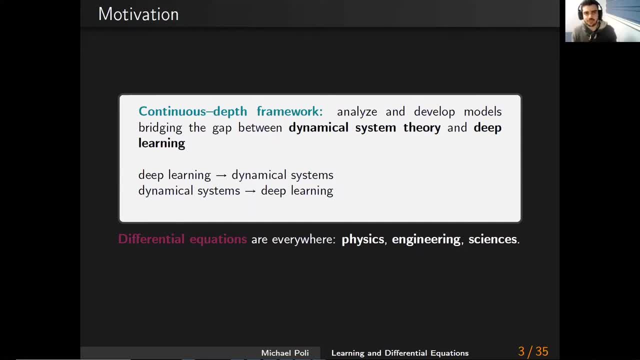 scientific machine learning, stuff like improving numerical methods with neural networks, for example. Some other people are working on the other direction, importing some of the mathematical tools and knowledge which have been developed for the past two centuries- almost longer: dynamical systems, optimal control. 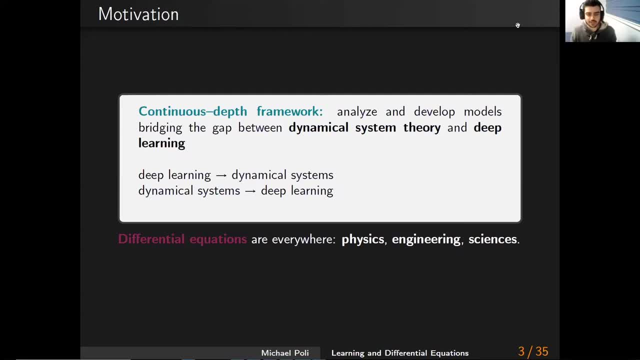 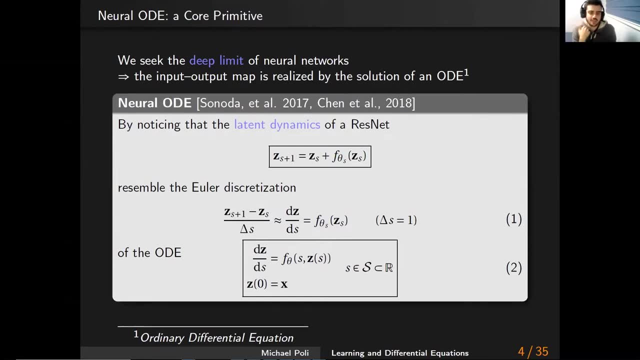 to help in more traditional machine learning tasks. So to start, let's dive a little bit more into the details and let's see how we can justify the formulation of neural OD, what the object is and how we can get there. So there's several ways to get to the neural OD formulation. 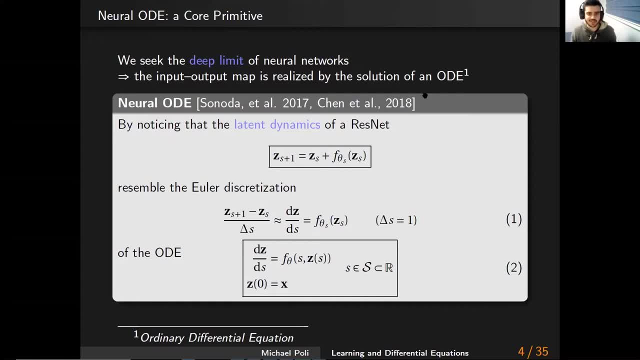 We'll take the say the original path of the seminal paper that I'm sure many of you have heard of, by Chen et al. the one best paper was one of the four best papers at NeurIPS 2018.. And the argument was as follows: 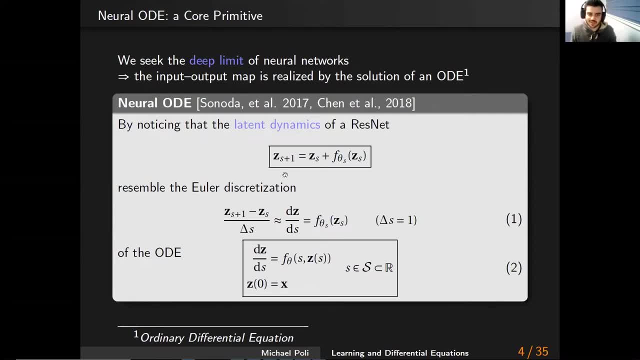 So let's say, let's suppose to have a discrete dynamical system of this type, which is indeed a residual network, So the layer to layer dynamics of the residual network, where you have the so-called skip connection, where you pass through a parametrized nonlinear function. 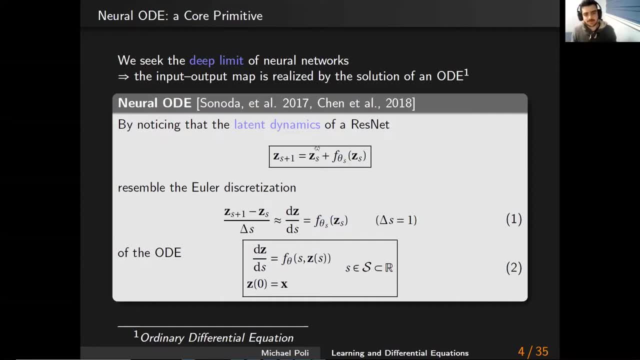 your residual block and then you add it back to your input. Now, if you squinted this, you introduce a sort of a phantom term here that that's been simplified away equal to one. If you squint at this and rearrange some of the terms. 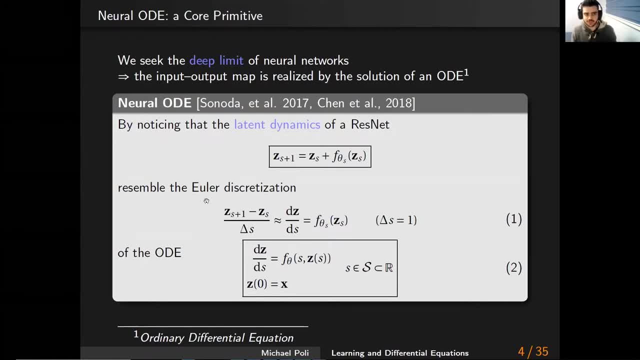 you see that it looks like a forward Euler discretization. for those of you that have a little bit of a background in numerical methods, or you remember calculus, It's sort of the definition of a forward derivative right, But we're missing the limit here. 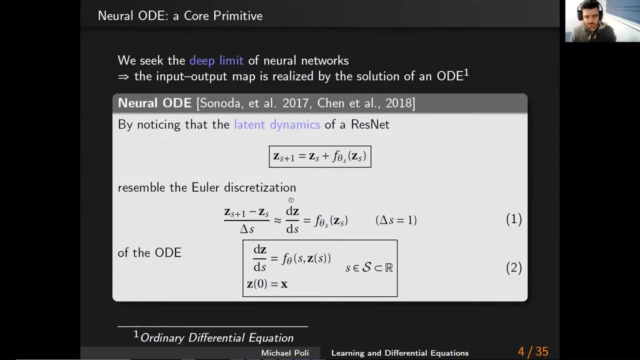 So it's sort of a rough approximation, very rough approximation, of the derivative in S. Now if you take this quantity here, you put it here, we're almost there, in the sense that we need to make some considerations. First off, S. here I'm using S for a very specific reason. 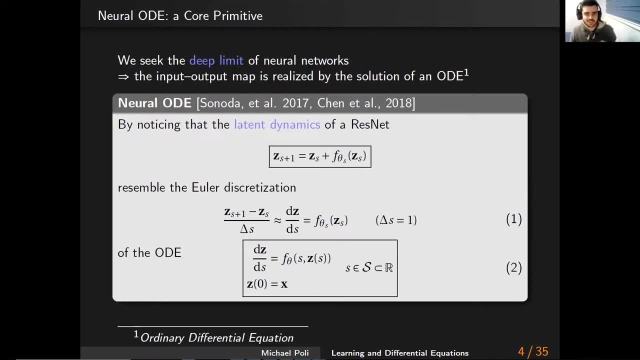 More traditional. you would use something like k to index, k integer to index your layer, layer 1,, layer 2, layer 3.. Now here S becomes a continuous, a real scalar value, And that's why it's called continuous stuff learning. 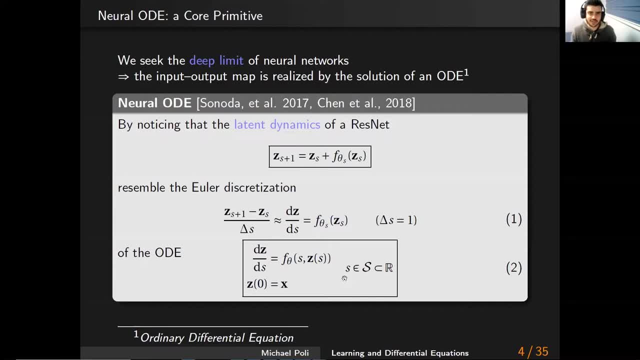 So you're still sort of indexing your layers, but you're doing it an infinite amount of times potentially. So that's the first difference. Second thing that's missing is an interface with the data. So we're trying to do learning, trying. 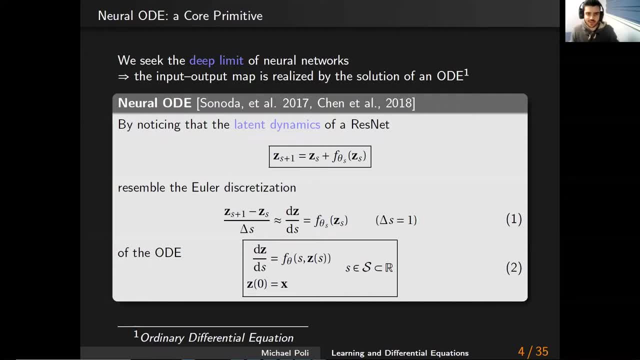 to achieve some task, to solve some task. So we need an interface with the external data, And the data for neural ODs is nothing more than the initial condition of this whole thing, which is nothing more than an initial value problem. So it's a problem that needs to be solved. 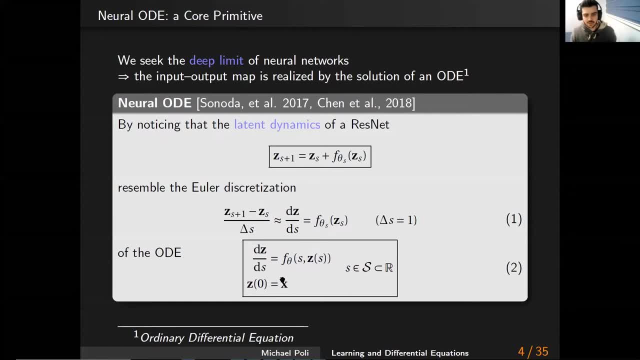 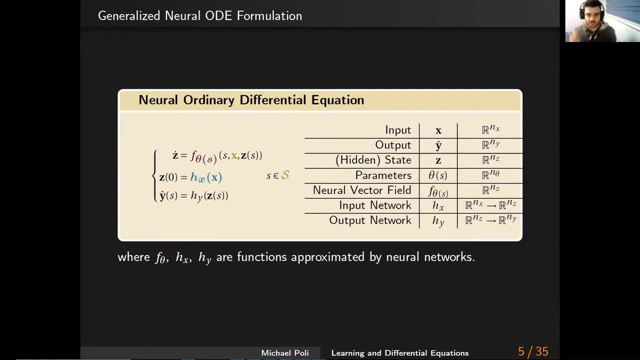 And this is where the numerical methods, for example, can come in right. If you add some more bells and whistles, this is the generalized formulation that you see in our world paper at NeurIPS. You might see some other things that 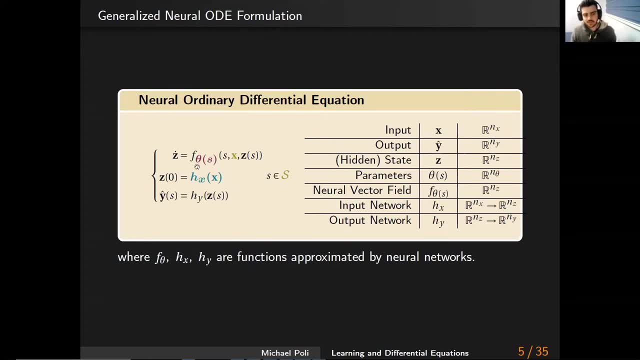 help relieve some of the limitations that we'll briefly see later. Something that's very useful, for example, is having parameters varying in depth. Now, this is where having the add s depth variable as a real really comes into play, right, Even in your residual networks, you 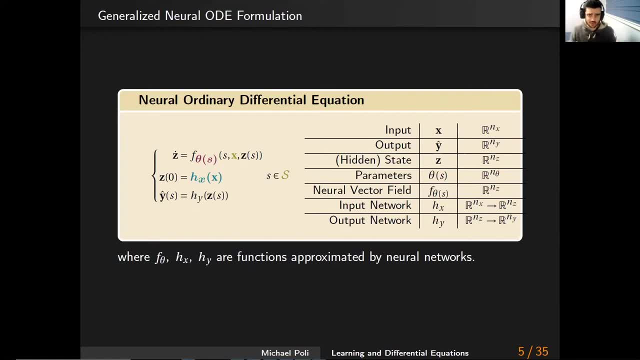 could think of the parameter tensors for each residual block as being a function, taking the layer index and spitting out your parameter tensor. You could think of it this way And indeed you can think of this. Let me open the chart, the other one. 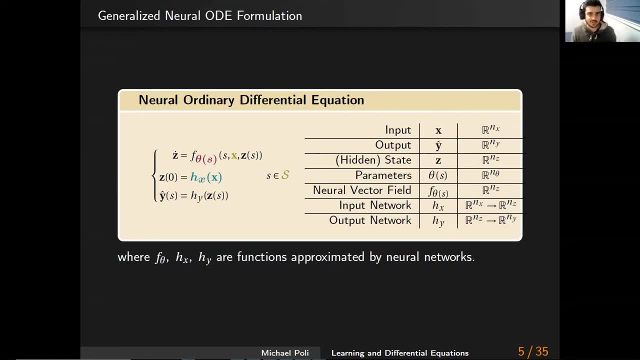 You can think of it even here in the same way. Indeed, here you have a complication: that you have infinitely many layers, And so if you have non-constant parameters, that's a problem that we'll see how to tackle. Something else you could have is a variable amount of depth. 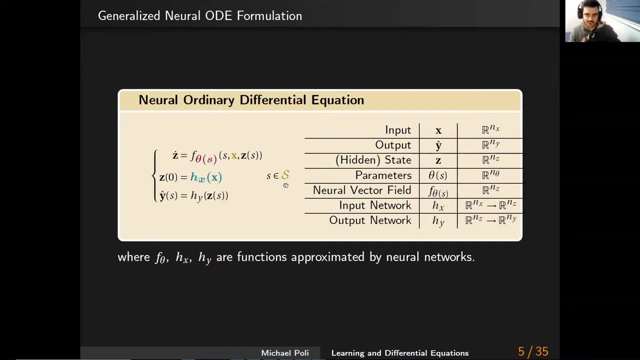 variable amount of layers. in some sense so a learnable integration bound for the initial value problem. You could have some embedding, encoding and decoding steps to go from your data space to your space where f lives And you can have some additional conditioning. 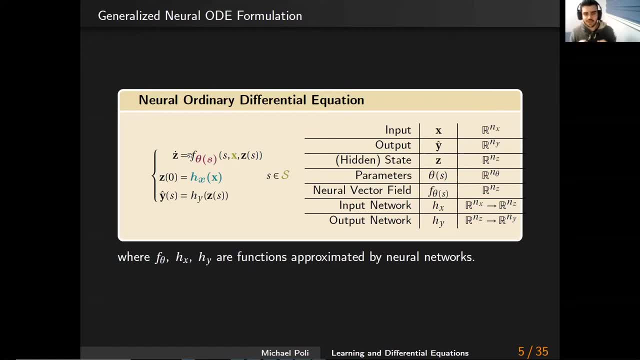 on the vector field. So the point here is f. f is everything. f is where the interfaces with neural networks. f is often a neural network parametrized by theta. It doesn't have to be a neural network, It can be anything. Gaussian process. that has been done. 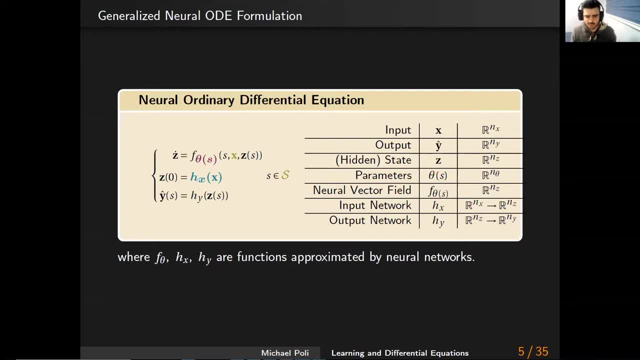 even non-parametric function approximators. It can really be anything. The point here is that By taking this view, we're transforming learning into a different type of problem, So we're learning the map directly that shapes the data in some way. 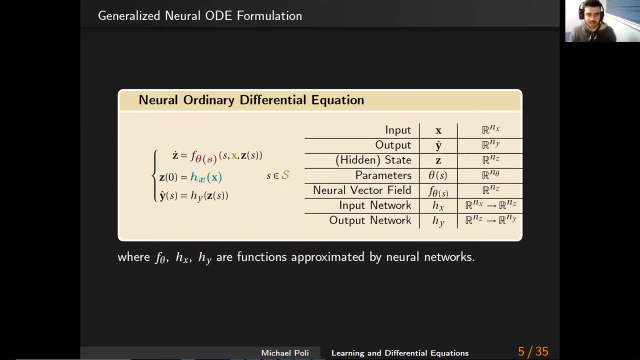 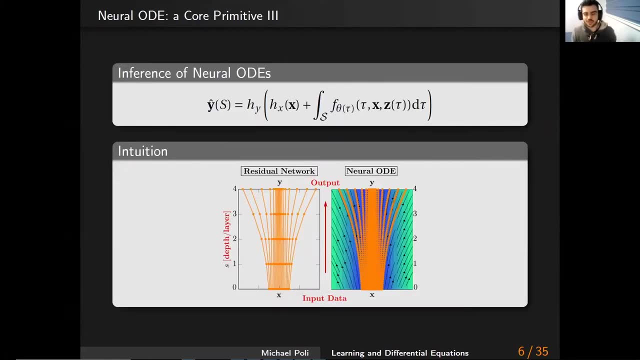 that morphs the data in some way. We're learning an underlying vector field that lives in some space, And I'll give you some more intuition later on. This is a good point to stop and really develop an intuition, which will then help pretty much everywhere. 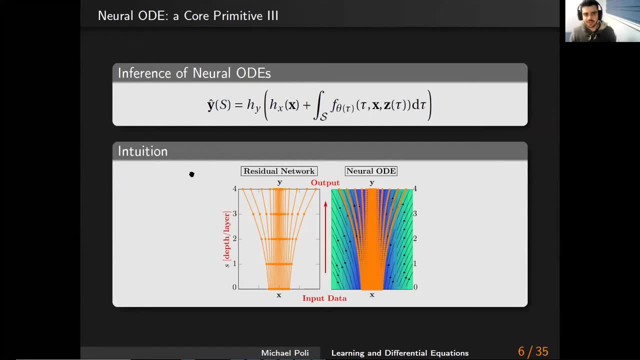 in this field. So the solution of an IVP? It simply takes this form: You have your input data, You map it to your initial condition, for example here. Now the problem is indeed here: solving for the integral of the vector field, which 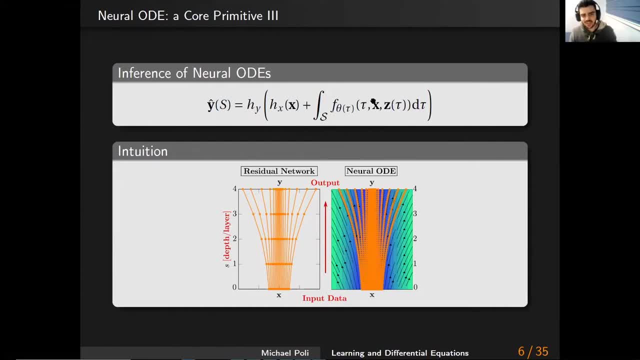 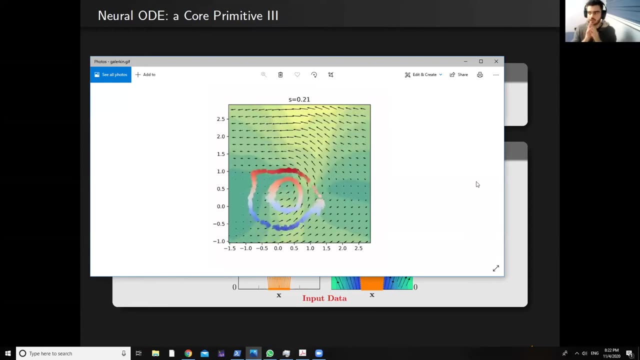 will draw this squiggly line. Then, taking the final point here, you can map it back with another neural network And you have your solution of the IVP. Now This is, I think, another very useful thing to look at. 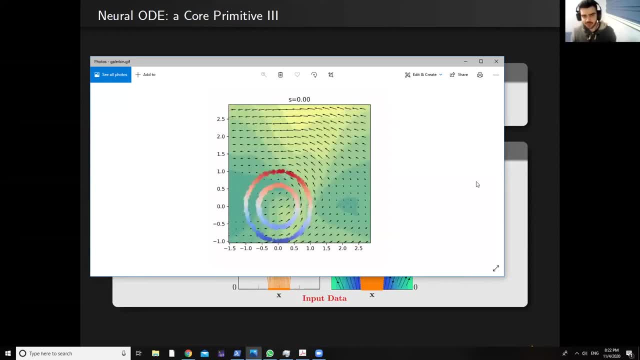 So what we are learning is a vector field, that is, a vector-valued function which takes. So we're living in some space of fixed dimension. We can change our dimension, So there is no, you know. and then linear, going from 10 to 15 to 10 to 4 across the neural D. 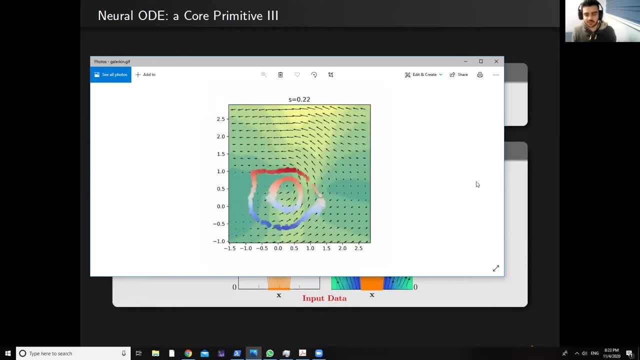 has to be fixed, sort of like a residual network. The vector field has to be shaped. So the vector field is parametrized. You see, it evolves both across training iterations as well as for depth varying parameters. Also varies across integration. 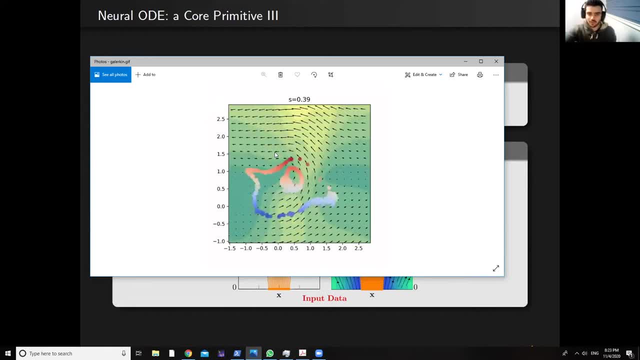 And it will learn to be shaped to pull data in certain ways that help for the task at hand. In this case, you're looking at the binary classification problem. We're trying to separate inner and outer circle And you see that the vector field 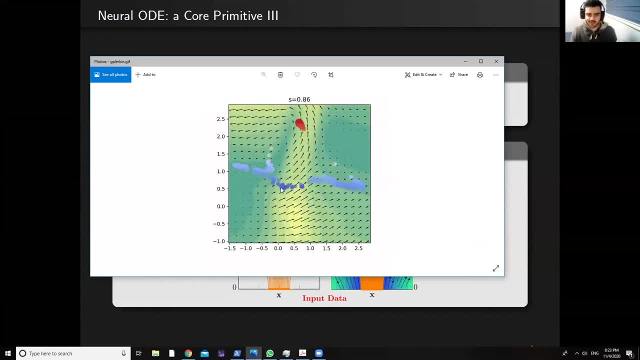 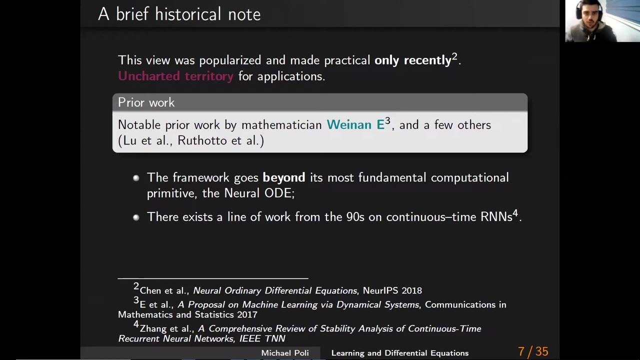 pulls the inner points apart. It even learns to flip it, to flip some of the vector field vectors to better help downstream layers achieve their task. So this is all the intuition that's really required to understand what is different about neural Ds. I'd like to say that there is, like I mentioned before, 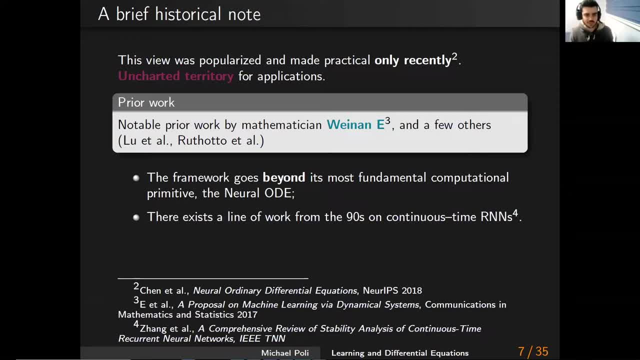 there's a long history between differential equations and machine learning. Even the idea of neural D itself- some would say the idea was in the air already. Indeed, if you check some of the work by a mathematician, Wayne and E and some others, you see that you. 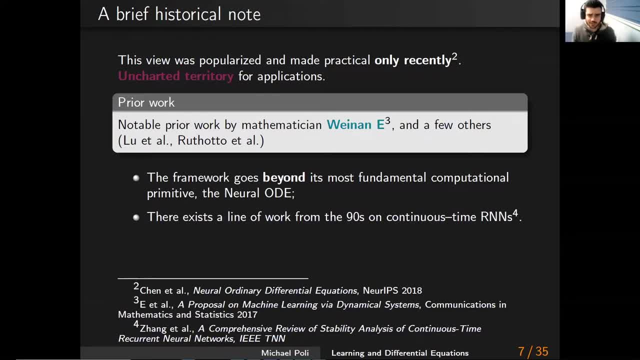 find some of these formalizations available, as well as the idea of normalizing flow, continuous normalizing flow as a link to optimal transport, for those of you that are familiar with normalizing flows. And there's also an even older line of work. 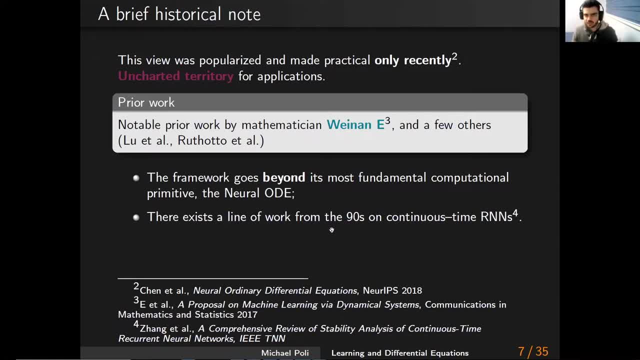 on continuous time. So the concept of depth and time is interesting. It's interesting to keep in mind. There's a difference. The reason why we use depth is that, for example, in a classification task, we are fixed in time. There's no time evolving. 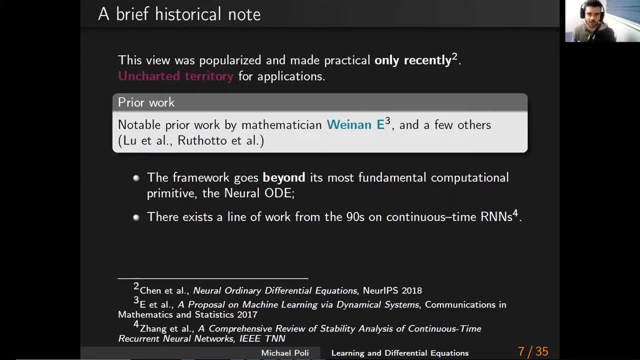 Depth takes more of a space connotation, so, evolving through the depth, the space of the network, You can view time. if you have a time series like an RNN, Then you can have the data time as time, the data dimension as time. 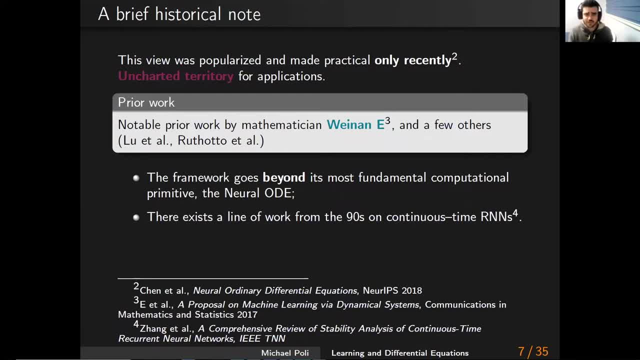 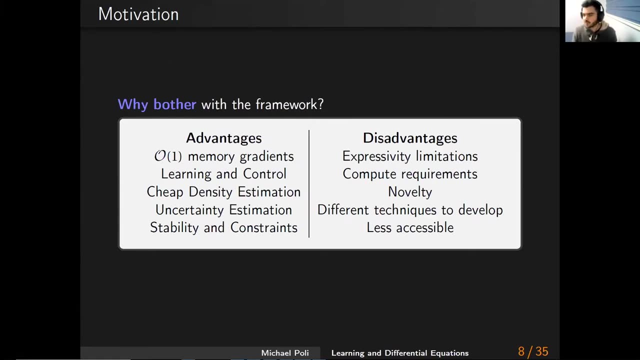 Or in some other references. you see the training iterations as time. So the vector field evolves in time. but solving on the vector field would be a propagation through depth of the network. OK, so why should we bother with this? There's many ways. 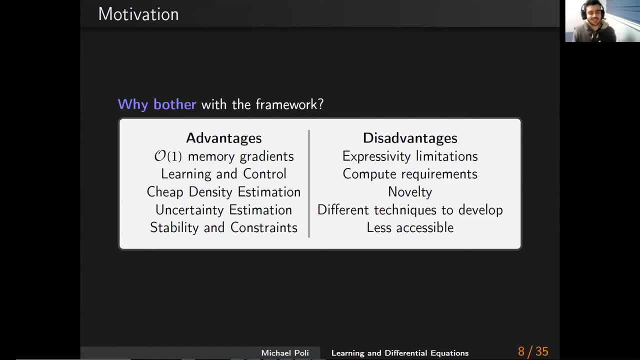 There's many aspects, many reasons for this. I'm going to be giving you some. Maybe some others will come up in the Q&A. So we'll start with say the reason that many think was behind the paper getting really popular. 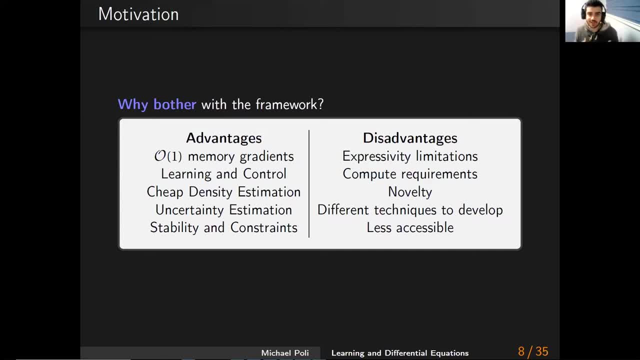 was this idea of having constant memory gradients, parameter gradients to optimize in standard deep learning fashion, and constant in depth. So in number of layers, on integration depth, we don't have any overhead. You have advantages in learning and control. It's a good prior knowledge to assert. 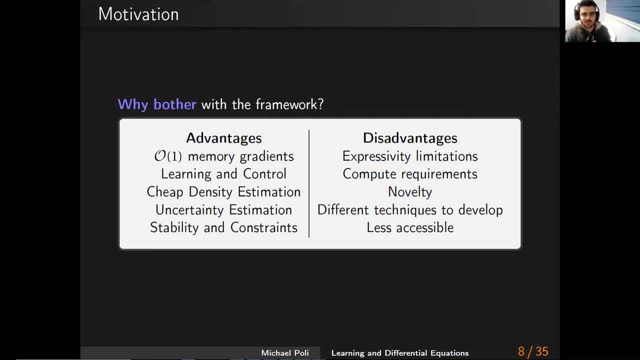 if you know you're controlling a robot, You know you want to use an OD. You even know a specific form of OD you might want to use. You might want to use an Euler-Lagrange formulation. You might want to use a second order system. 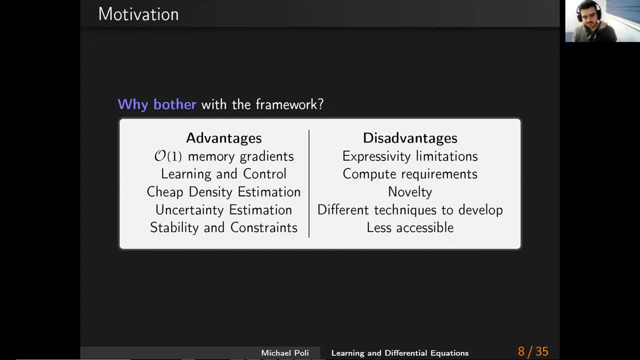 if it's mechanical, et cetera. Similarly for forecasting. if you want to do stock price forecasting, you might want to use a neural SD. You might have some prior knowledge on all kinds of parameters that you can include. You can do a cheap density estimation. 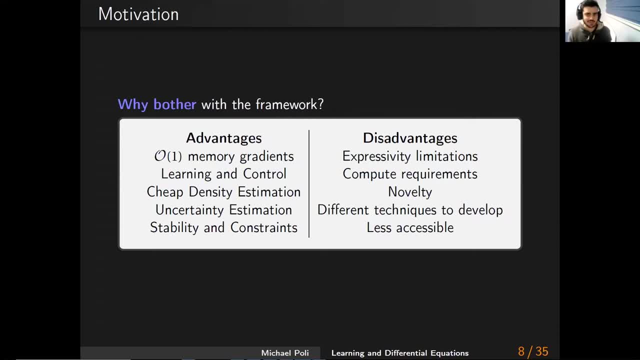 You can do other things. Now there is also disadvantages that are important to keep in mind. So neural IDs are less expressive- unless you're careful about how you design your model- than equivalent or analog discrete models. They have more computer requirements. 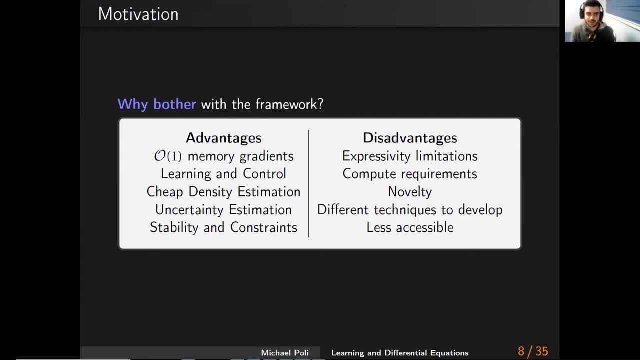 because it's no longer only about the model, but it's about the model and the solver. We'll see this later with the hyper-solver idea. It's new, So there's different techniques and mathematical tools to develop, to use in order to fully understand. 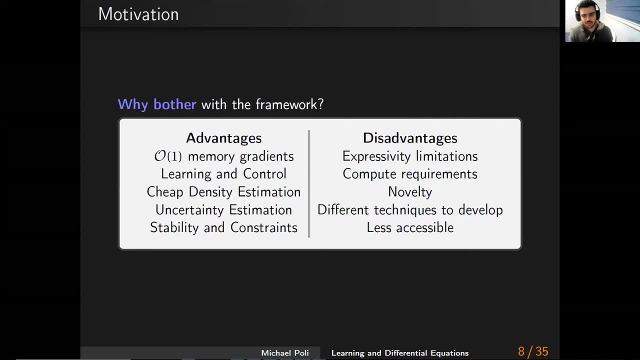 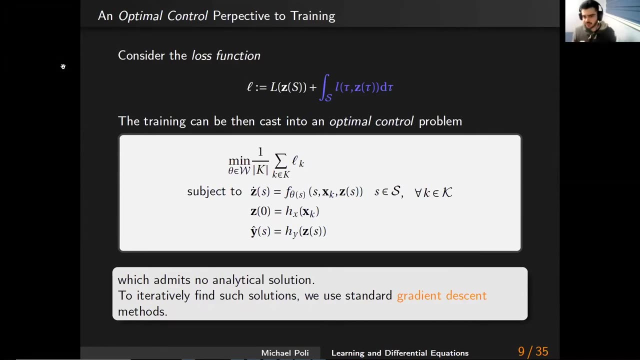 And implement- even implement on a practical level- these models, And thus it's less accessible. I hope the talk today will be a small remedy for the last advantage. So we start with the most technically involved section. I don't expect all of you to understand all the details. 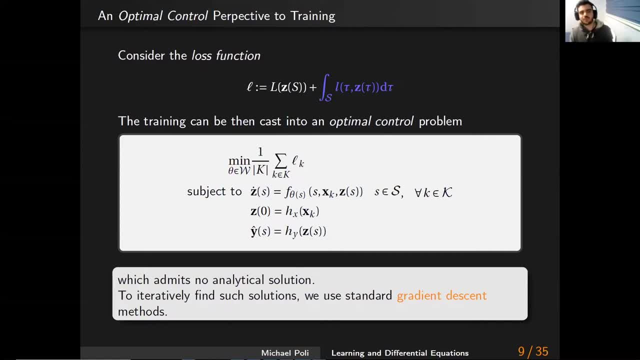 unless you have prior background on either optimal control or really excellent background on ODEs, And I'm going to be giving you a proof sketch of some of the intuitions. hopefully, At least you have an idea of how training is performed for these models. 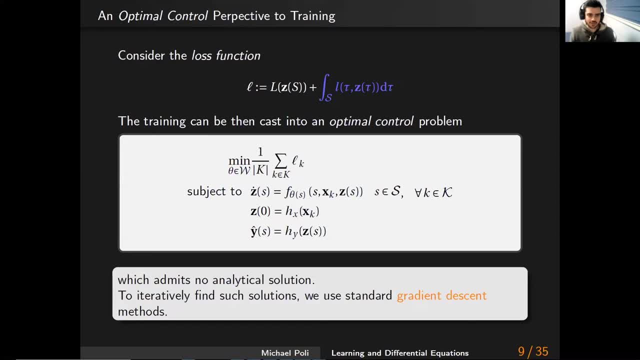 So let's suppose to have a loss function of this type that has two terms: a terminal loss term or, for those of you from control, terminal cost. We assume to have maybe some downstream layers, right? So this is the solution of the OD. 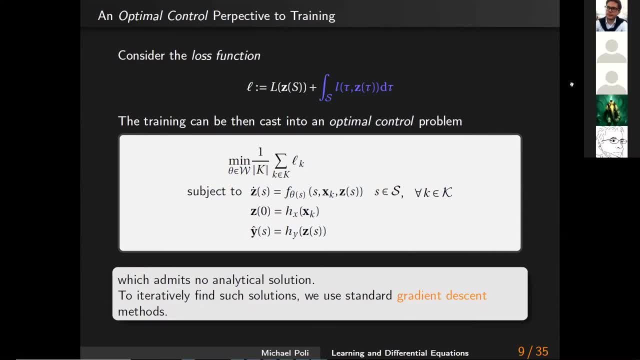 We assume to have the neural OD. So now, if you look at this, this is- and you're also familiar with- optimal control. This is the type of loss that you see in control And if you want to minimize this, what you're ending up with. 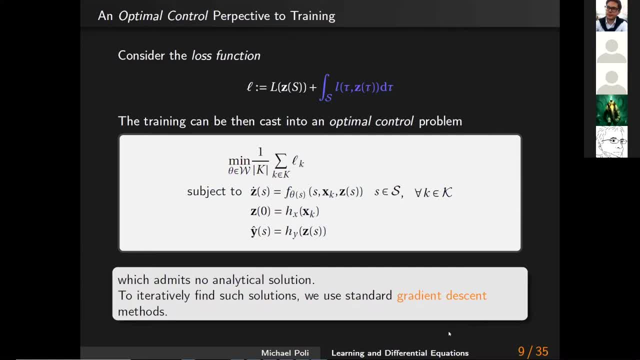 is an optimal control problem of this type, right. So the problem now I say the OD itself- becomes a constraint of the problem, trying to minimize this loss function. So what we're doing is that we have a very simple problem here. So we have the 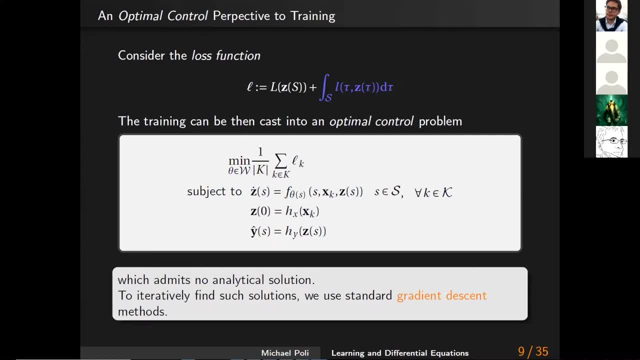 We can solve this analytically, but we need some assumptions on F, the dynamics and the constraint And in this case, where the vector field itself is a neural network, a really complicated function, it's impossible to to find an analytic solution, which means we're going to approximate a solution as good a solution. 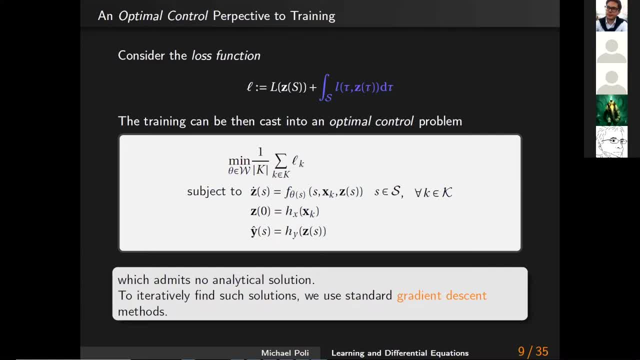 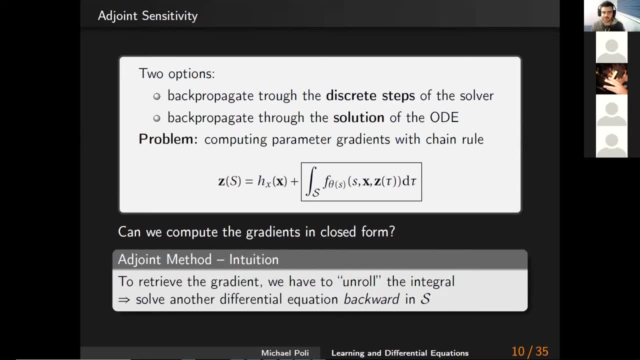 as we can find. so it will be a non-globally optimum solution with gradient descent, an iterative procedure and the parameters. so our task is finding these gradients. with respect to the parameters, as with any other learning task, we have two options, two umbrella options. one is by 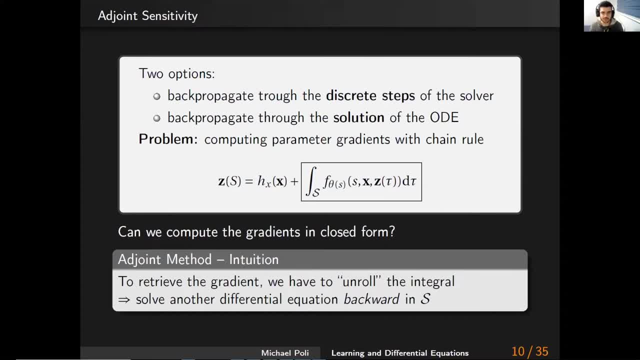 propagating, through the discretization of DOD, the solution of the initial value problem, which would be doable, right, no problem, we will choose a numerical solver, like the Euler scheme that we saw before, which approximates this continuous solution with a limited number of steps. this is: 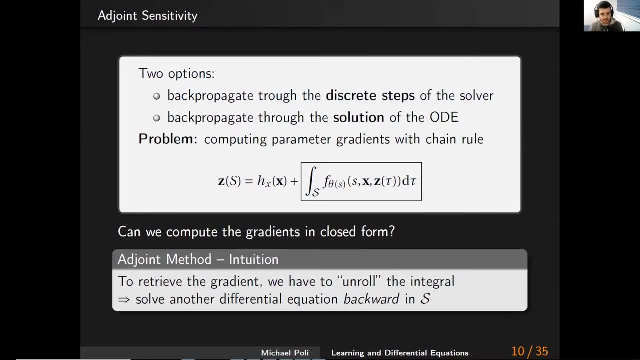 what you will often do in implementation, but it's not the actual gradient with respect through the solution of the second option is you have to find a way to do this in closed form, analytically for the gradients with respect to theta or the loss with respect. 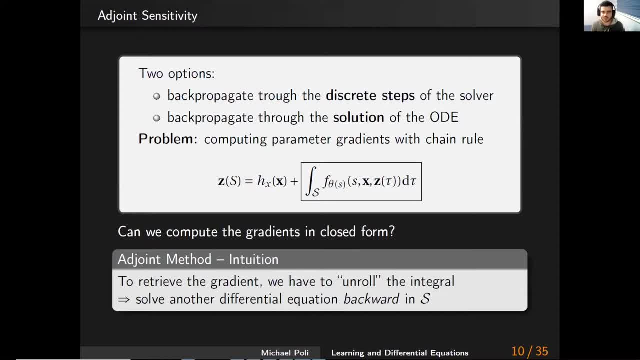 to theta and the problem of using your traditional chain rule is this integral right here that poses problems. so here comes the like, the joint method comes to the rescue and though the way it works is the intuition is, we introduce an additional set of variables, a cost state. 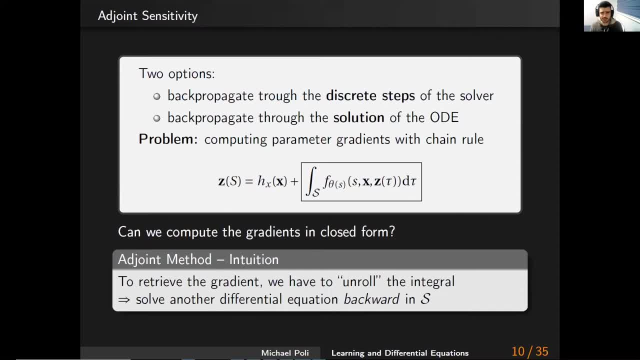 back of Lagrangian multipliers. so we're applying some ideas from the calculus of variations and we're solving another ODE. right, we're solving a final value problem because we have a boundary condition at the end of the network, the final depth, when I'm running it backward in such a way. 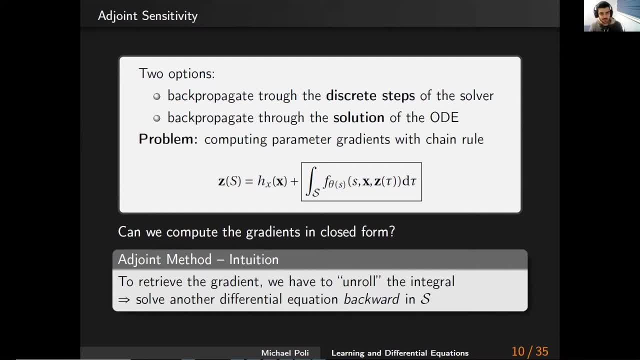 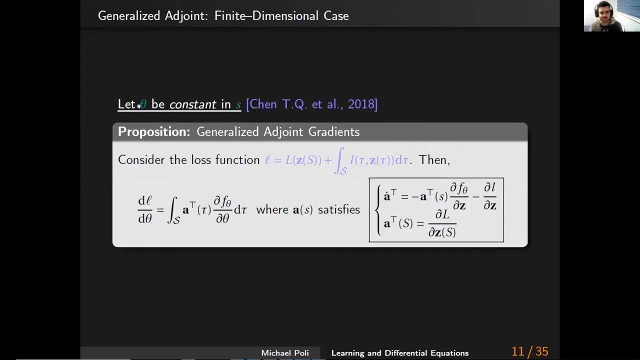 so that the a's will be defined in such a way that we have a specific relationship that defines our gradients in particular. this is what it looks like. so, for the simplest case where parameters are fixed in depth, you have your optimal control problem. this is your final value problem. a is your vector. 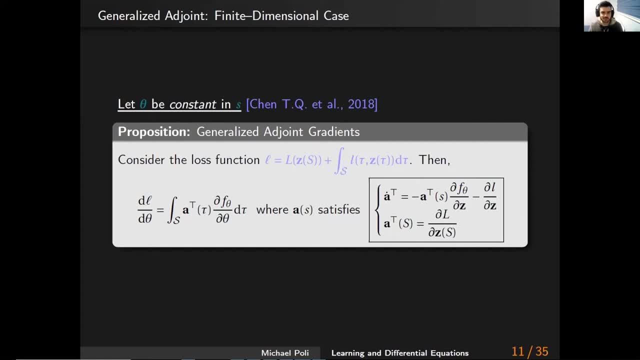 your costate vector, your vector of Lagrangian multipliers, depending on what your say perspective is on this type of approach. this is what it is and you're essentially saying, if my a starts, so the initial, the final value, but the initial value for the backward to d. 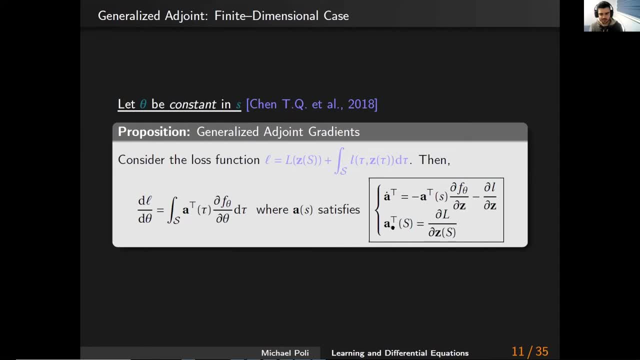 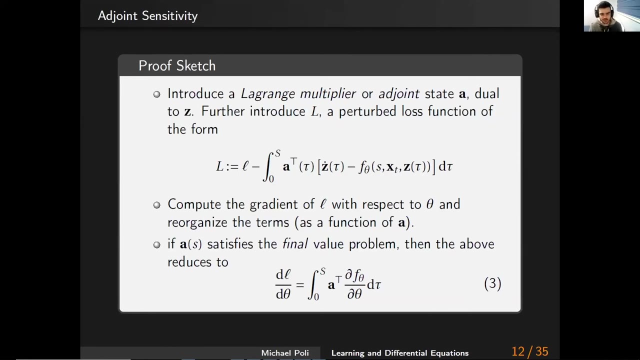 is the gradient of this terminal loss with respect to the solution, and it evolves according to this relationship. here Then I have this closed form expression for the gradients. So the proof sketch Now fully diving deep into this will require another 20, 30 minutes. 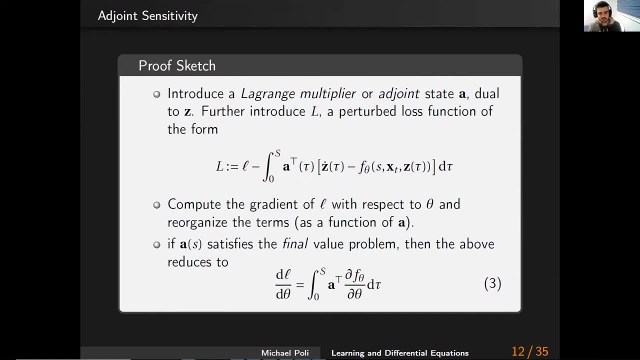 I will give you a proof sketch to get you thinking about. maybe you have some other perspectives that you can connect to this, some other proofs, some other ideas that you've seen, If you're really serious into doing research in this field or you're just interested in getting your hands dirty. 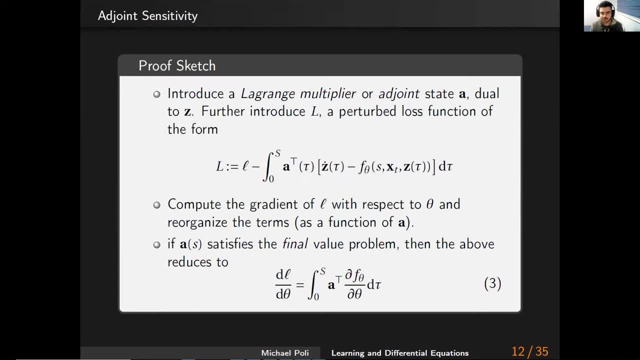 I suggest walking through this proof yourself. It's maybe 10 lines, so mostly rearranging terms. We have a good preference, I think, in our paper, in the appendix, very compact proof And the proof goes as follows: It's a few steps, conceptual steps. 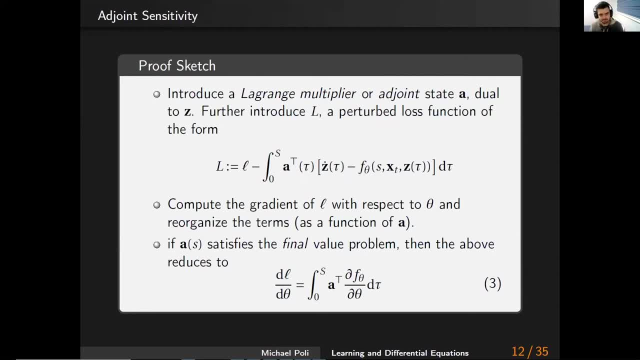 First introduce Lagrangian multipliers. So you have to introduce a perturbed version of the loss. I think in this way, As in traditional calculus of variation, your Lagrangian multipliers will be weighting the amount that you're not respecting your condition. 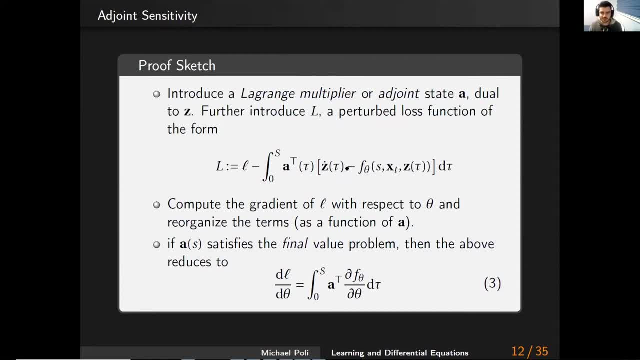 your constraint, This is the. if you put an equal here, you recall this is the dynamics constraint of the optimal constraint. This is the normal control problem. L is your total loss. So you're introducing a perturbed version of L. Then you're computing the derivative of L. 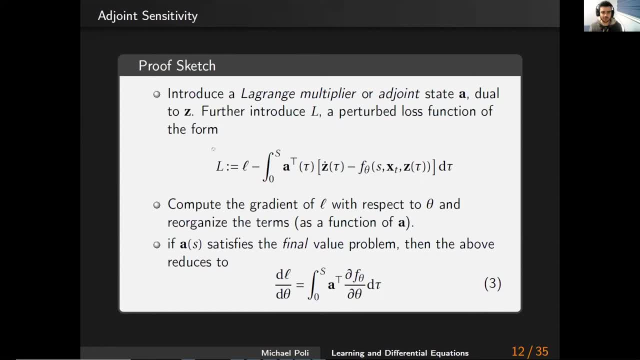 with respect to the parameters As a function of A. you flip this to the left side and then you'll do a little bit of integration by parts And there's a couple of steps. You get a function of A of this Lagrangian multiplier vector. 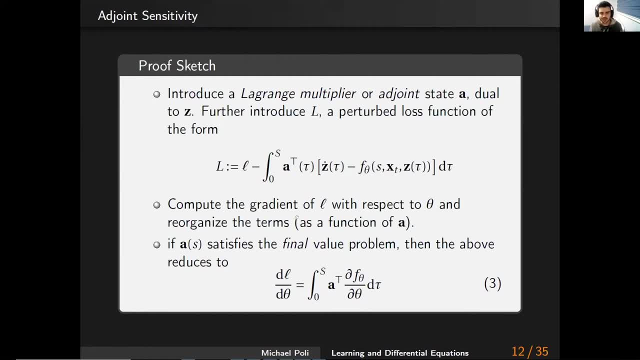 And then you pause it. You say if A satisfies the final value problem that we saw before, then you can simplify a lot of terms away and you get this. So what you calculated in the second step simplifies in several ways and you get this form here: 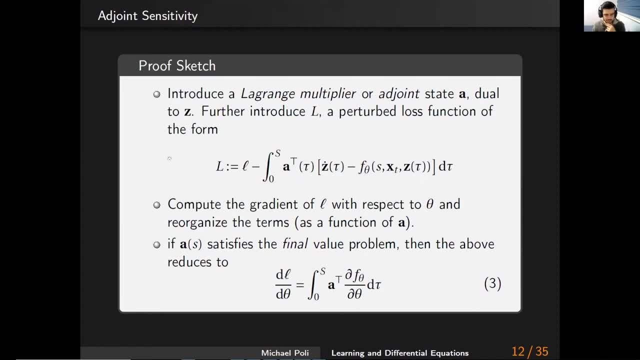 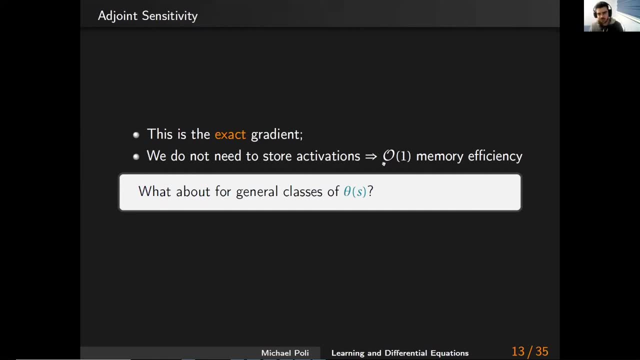 which is easy to compute- easy enough to compute in your preferred deep learning frameworks. So this is the exact gradients. What do we do? We don't need to store anything for this. What do we do in case the parameters are a function of S itself, so they're not constants? 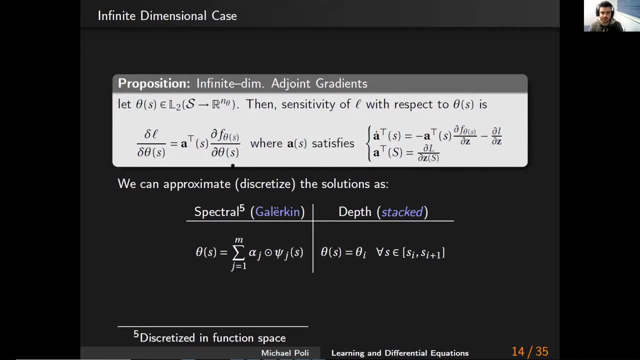 Well, in that case you need to go a little bit beyond what you saw before. This is also in the appendix of one of our new papers. You need to make some assumptions to simplify the proof at a couple of key points, in that the function theta of S needs to belong to. 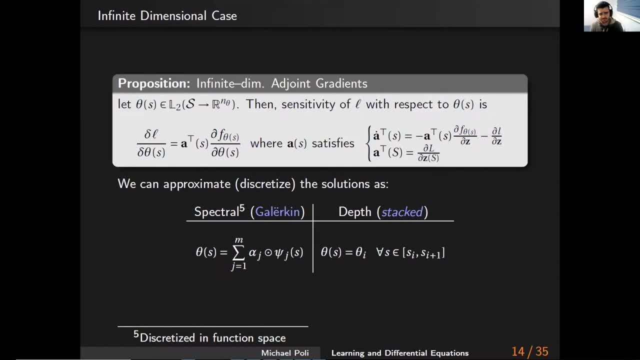 needs to be a square, integrable function that comes into play. We're simplifying with the Dirac delta, if you like, If you're interested in the details. But you see that this is exactly the same. You just change Here. you have a derivative in function space. 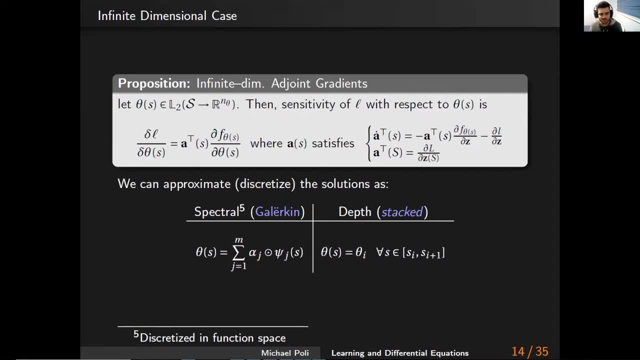 It's called gap-to-derivative function space, which is impossible or very difficult to compute, I should say. So you need to introduce another discretization, another approximation of the problem, to compute this, to actually compute this and implement this. 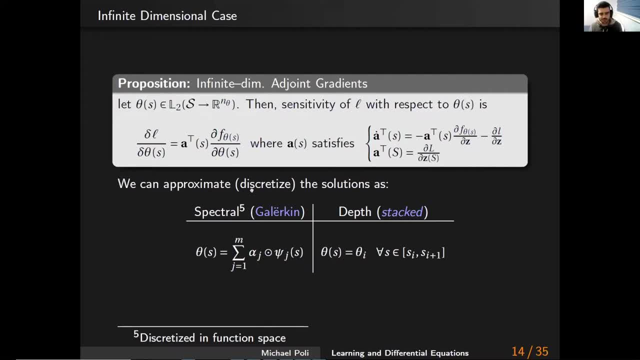 There's two ways, two main ways to do this. You can discretize in depth, so in S That means you have parameters that are piecewise constant And in that case- we saw before- you have just many of the same problem we saw before. 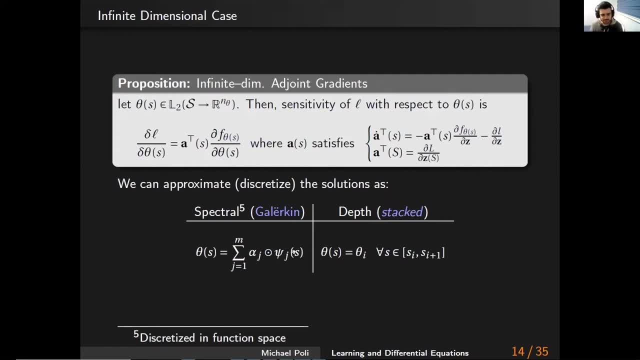 So you know exactly how to compute the gradients. Or you can discretize in function space, meaning you don't consider all square integrable functions, You choose a subset of them that can be expressed as a linear combination, the alpha j's of some eigenfunctions. 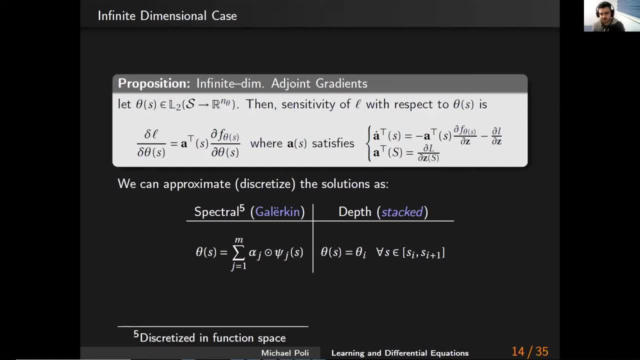 You choose an eigenbasis, So function that could be Fourier harmonics, could be polynomials, Chebyshev polynomials, And then you turn this into the learning of these alphas that combine your eigenfunctions. And this is what it looks like. 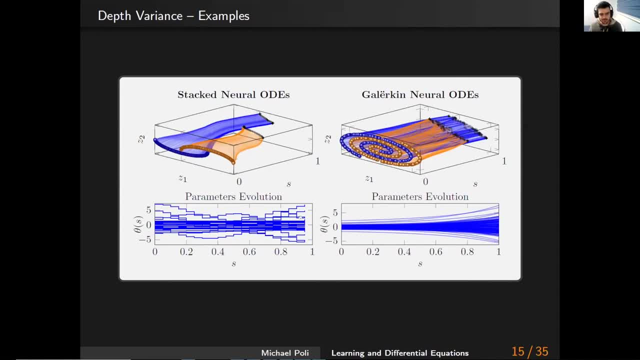 for a binary classification problem. You have a piecewise constant parameter, So you might have a polynomial discretization. So again, this doesn't look discrete. It's discrete in the space of functions, So it's less expressing the space of functions, but it's. 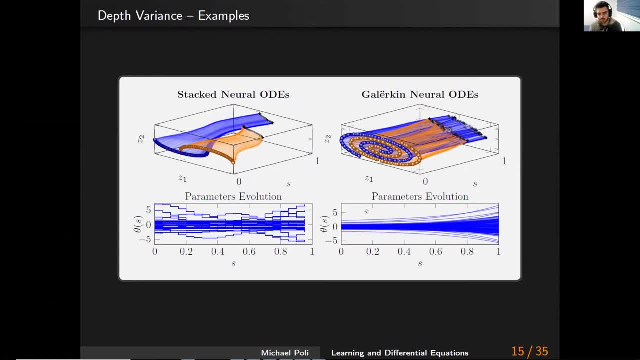 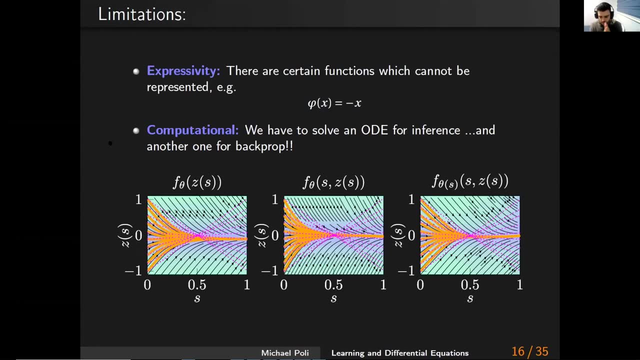 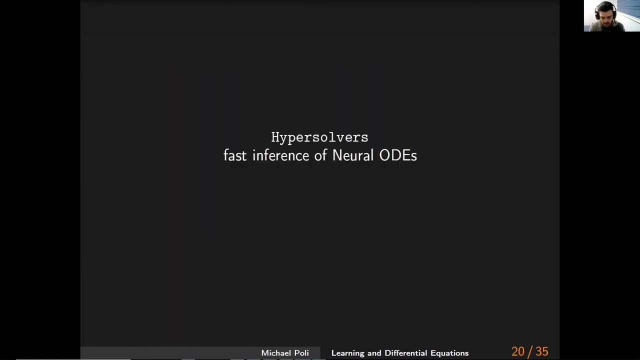 it's continuous in that right here, And if you, if you use Vanilla NeuroDs, you would have a constant functions here. Okay, So let's move along a little bit, I think to here. So there's a lot more to say about NeuroDs. 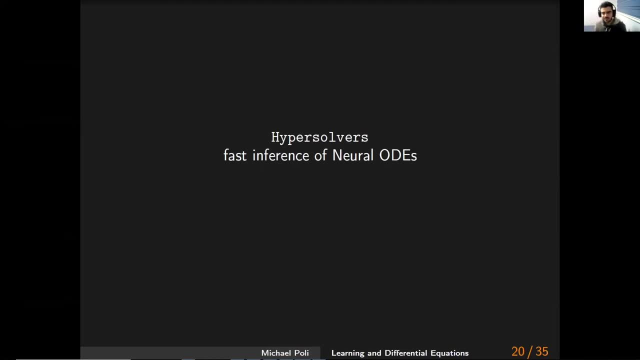 It's arguably one of the hottest subfields now in deep learning, At least in some key conferences, And for good reason, like there's many applications are. pretty much every week there's a new paper exploring a new application And you know it's. it's an attractive way. 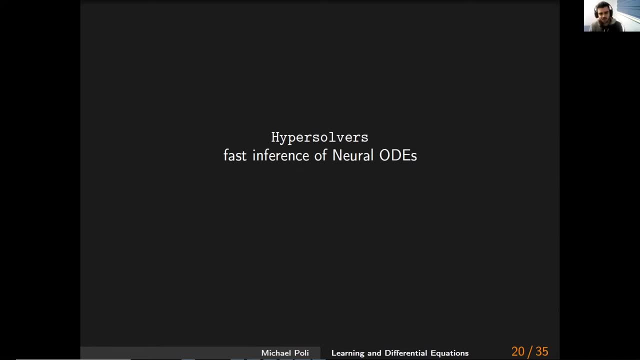 to impose your prior knowledge of the model. Why should we do reinforcement learning with RNN, surrogate models when we can? we know we're controlling a pendulum, for example, We know exactly what shape DOD has, Even if we don't know every parameter. 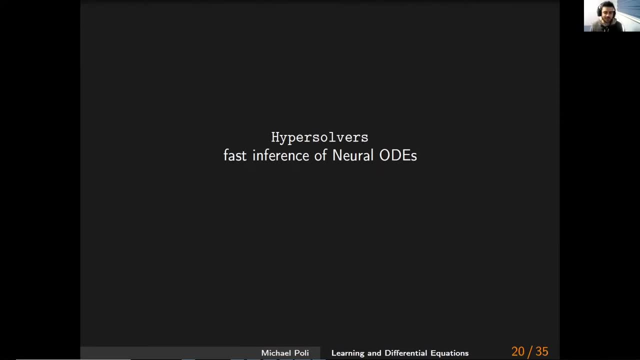 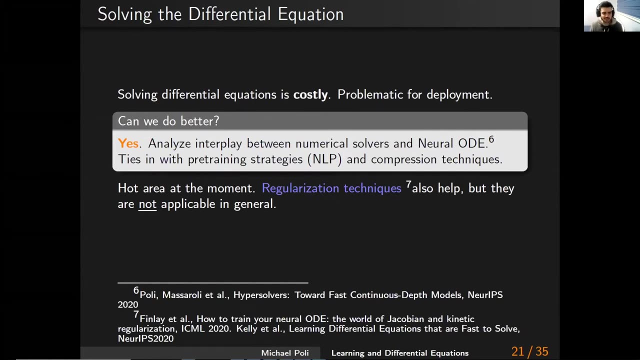 we know more or less. you know, might know it's conservative, we might know So it's. in that sense it's good. What are the downsides? The downsides? it's, there's many, as we saw before. 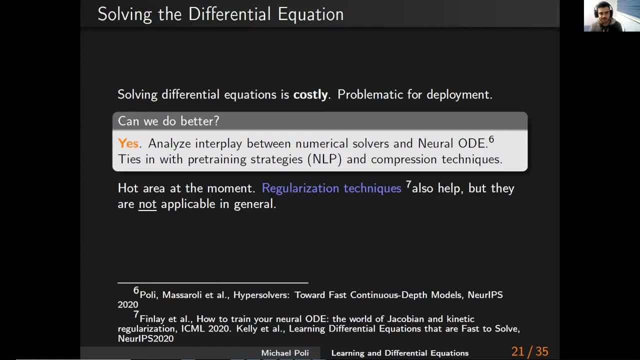 The greatest one that's currently slowing the field down is the fact that these are slow- slow for inference And for training. the problem is is related to the inference speed. In terms of training iterations, they're often better than corresponding analog discrete models. 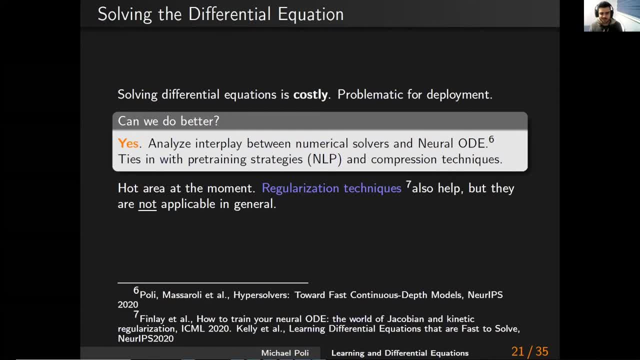 It's just that to do one inference pass, it takes longer. If you need to choose a solver, you need to choose a correct solver. You need to ensure that the solution is close enough and can be difficult, something that people are studying, thinking about. 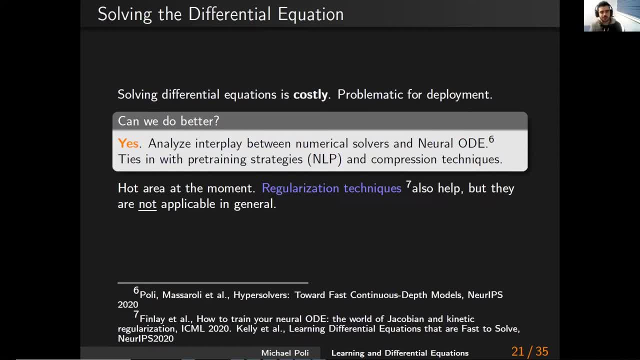 is regularization techniques for the vector field And it's a. it's a strange regularization perspective in that we're trying to make the vector field easier to solve, for usually adaptive steps solve. So we're trying to make the vector field less nonlinear, less, let's say, more well-behaved. 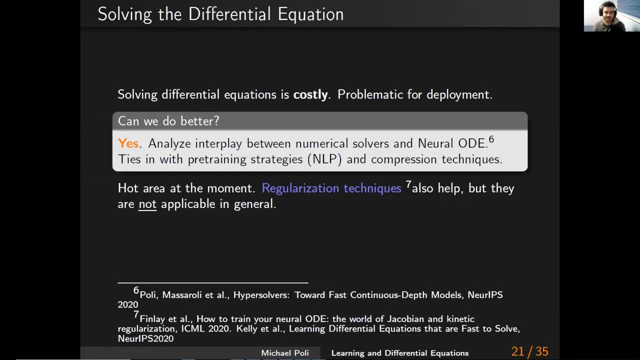 so that it's easier to solve, but then in some perspective it's also putting some constraints on the expressivity of the model. So similar to your L2, L1 regularization, but more indirect. perhaps Now what the problem is with these approaches. 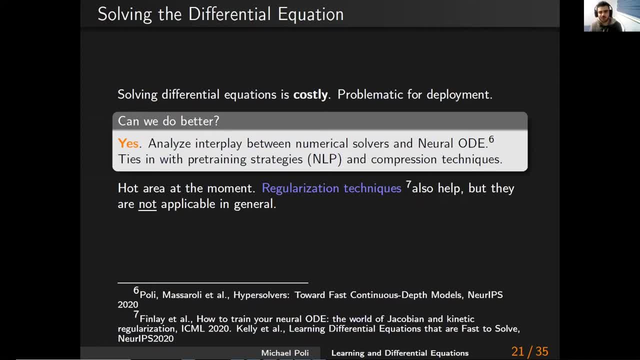 is that you can't always regularize the vector field. So if you're doing control and you have a partial model of your robotic arm, there's nothing you can do to regularize the dynamics of your robot. You know they're what they are and often ugly. 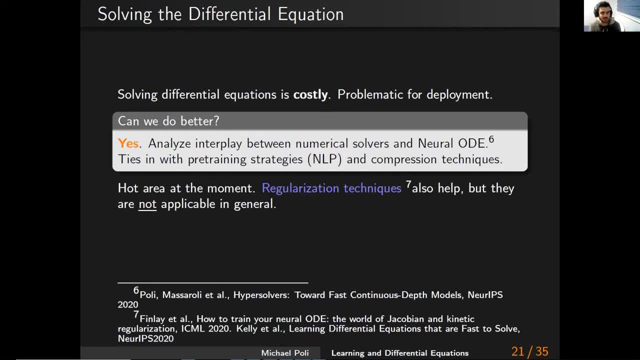 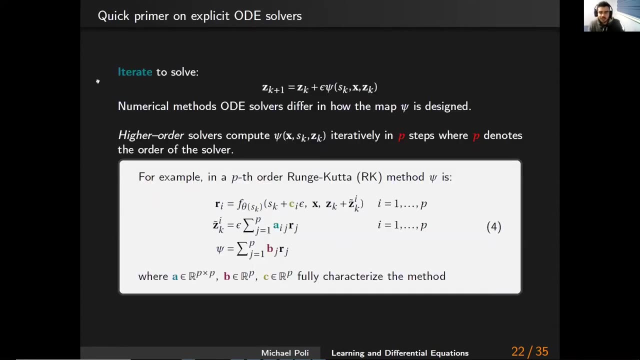 So this is not the answer. going forward Probably won't be the answer for all applications. It's pretty good for purely machine learning applications where you don't have any other prior component of the OD or DST or whatever. So what we would like, then, is to explore the connection. 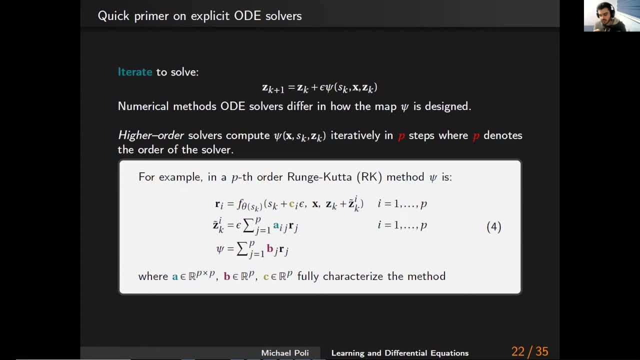 with solvers, like, instead of taking solvers as another black box component we're just importing into our field, We want to look at them as design components as well. So how to make this interplay better, how to understand it better? 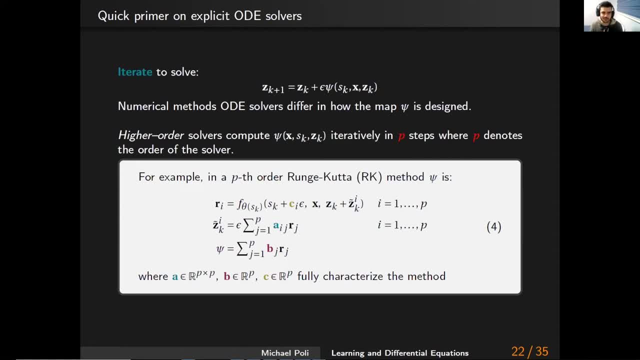 So very quick primer cause. we don't have a lot of time on OD solvers, explicit OD solvers. So we saw the Euler forward method. you're just iterating through the integral to approximate it as well as you can. right, You're choosing some points on your. 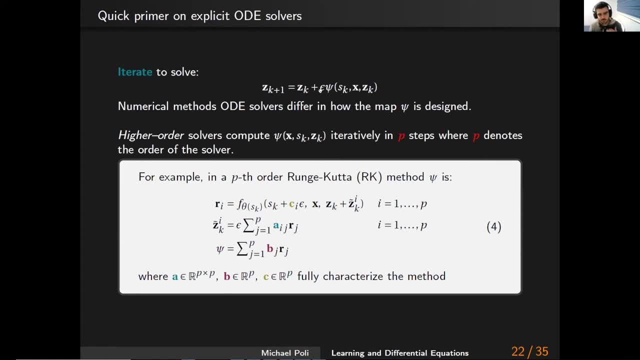 on your continuous solution. Your design choices are your, your step size, your map fee. So for Euler, I should say for Euler, it's simply the vector field evaluated at that point. for other solvers, such as Runge-Kutta methods, which are really popular, 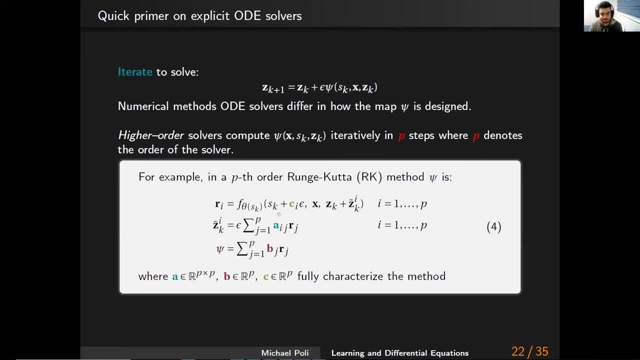 It's a combination of various things. The quickest way, the most complete way you can characterize a method is by the Butcher-Tableau coefficients. These are coefficients that are collected in a certain way, displayed in a certain way. There's a matrix A. 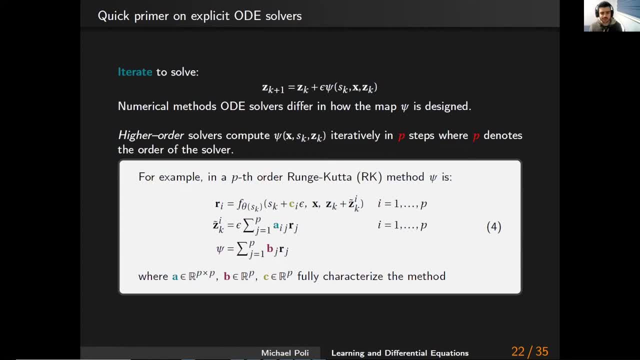 and there's two vector coefficients And these tell you how you you combine certain stage evaluations of the solver. They're found in very specific ways. So the field of numerical analysis, This is often, this is what a lot of it is trying to improve, trying to find better coefficients. 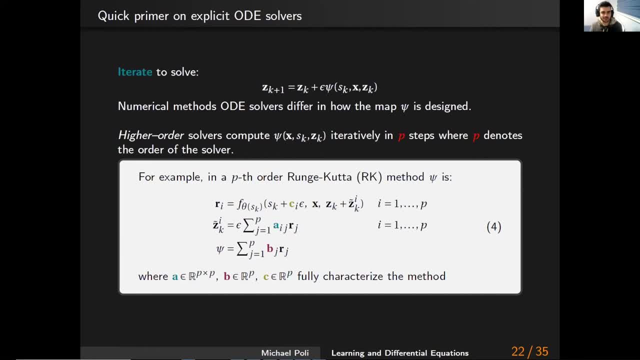 by solving different optimization problems, So putting different constraints on the type of solver you want. you want to get better coefficients And different solvers have different properties. of course, This is only a very small fraction. There's multi-step solvers. 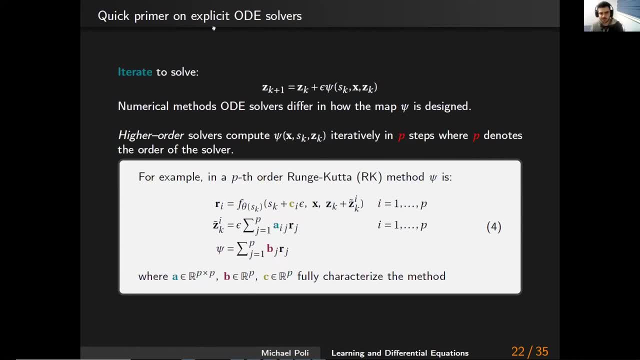 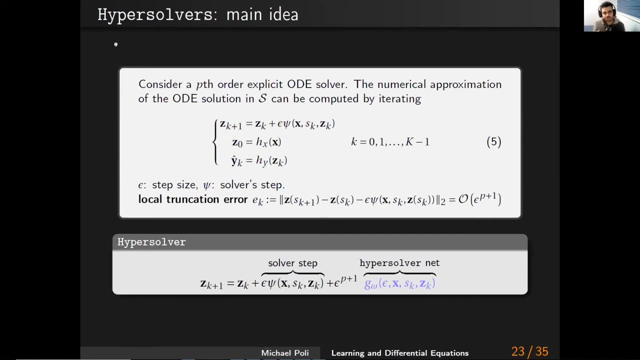 there's predictor-corrector schemes, adaptive step, implicit, et cetera, But this will do for the discussion. So the upper solver idea, what we would like to shine light on is the fact that you can discretize a neural OD. 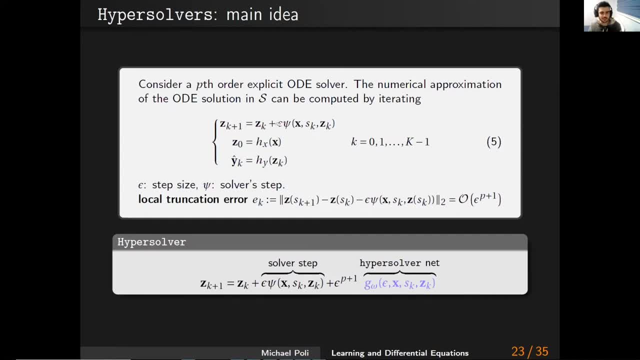 You need to discretize a neural OD to solve it. We'd like to have a faster neural OD- that the number of discretization steps for an accurate solution needs to be minimized. So how should we do this? A way is to take the solver a pth order. 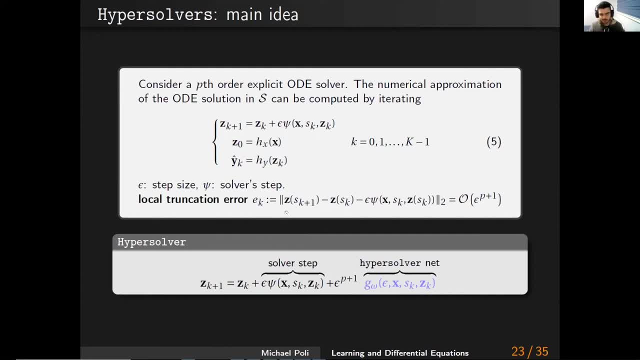 and the hyper solver, which means we're doing p roughly speaking. there's some technicalities involved. we're doing p evaluations of the vector field. so if the vector field is 10 layer neural network, you want to minimize that as much as possible. 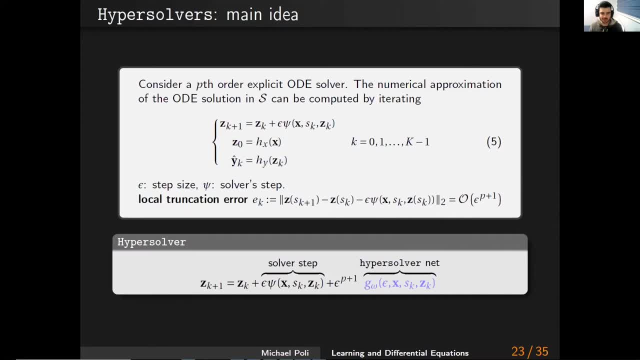 For one step of your approximation, your discretization. you're doing many evaluations, many forward passes of the vector field, the neural network. So you want to take a base solver, pth order, and you want to make it better by introducing a learning component. 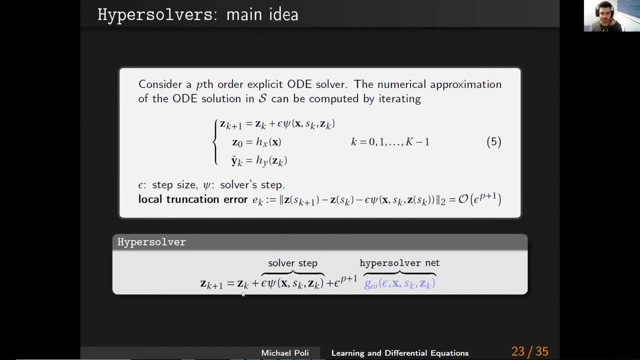 and hypersolvers network, so we call hyper solver this whole combination. the upper solver is trained on local truncation residuals. so you're you're looking at your discretization of the base solver and then at each point you're comparing the step that would be taken by the solver and one taken. 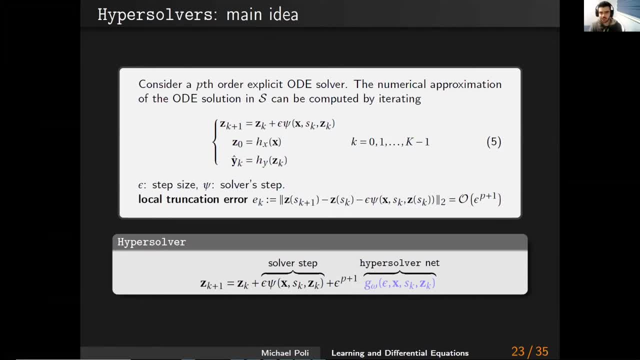 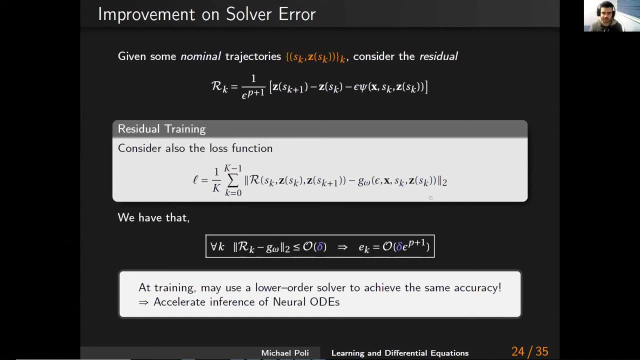 by a really accurate solver or the actual ground truth solution, if you have it available, if you do this, so you solve this, this supervised learning problem or g, and you have this better bound on the local truncation error, which is better than your, your. this is the step size by: 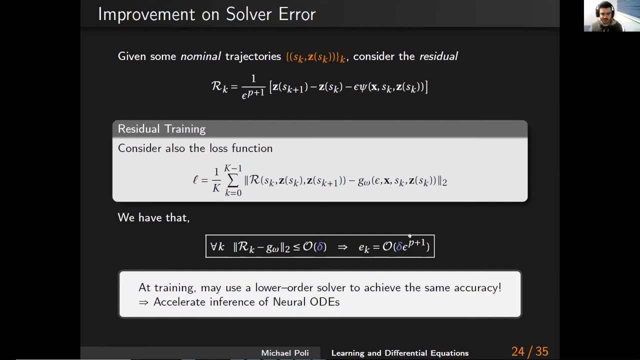 the way you would have an epsilon to the p for the pth order solve and instead you have a delta epsilon to the p plus one where delta, if delta is the, the approximation capability, like your hypersolver is the approximation capability of the network. uh, if you train you correctly, will be an epsilon, will be a delta approximator. 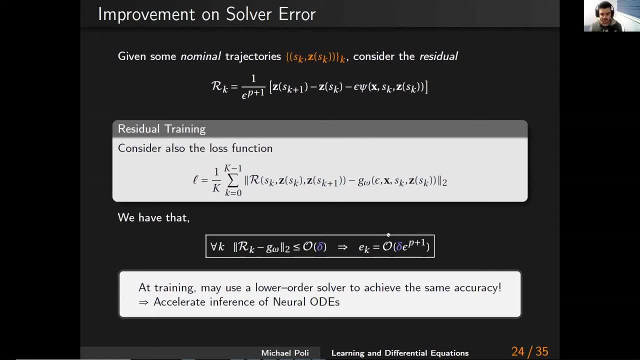 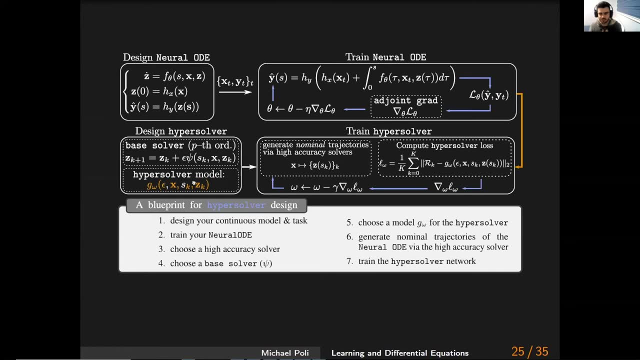 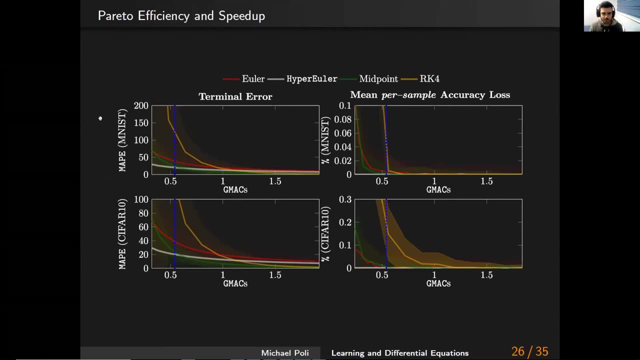 where delta is hopefully much smaller than one. so you have a better um, a better bound here, um. this is a good reference if you'd like to have a clearer picture of how you can do this when you know these and um. you compare this with other solvers, even higher order solvers. so say we have. 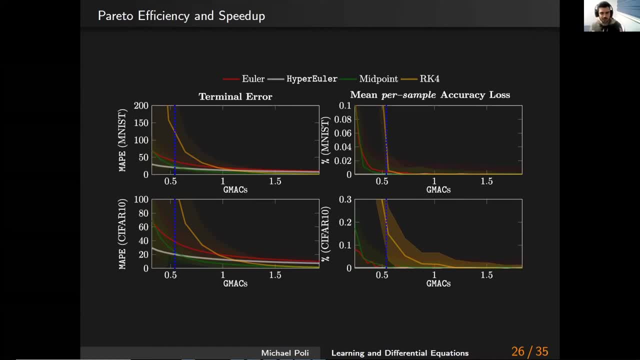 an hyper euler variant. so it's a. it's a first order method with a learning component to approximate second order residuals- you are more competitive than your, your base solver- but also higher order methods, and here you're looking at first row, you're looking at mnist results for a neural d image classification. 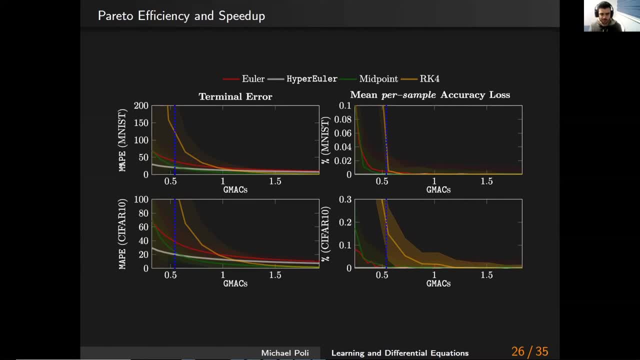 cipher 10, you're looking at solution error, average percentage error on the actual solution. you don't care about about the task. and here you're looking at test classification accuracy. so you're training with an adaptive step solver that's really accurate. and then you you're evaluating how much you're losing by then speeding up for inference later. 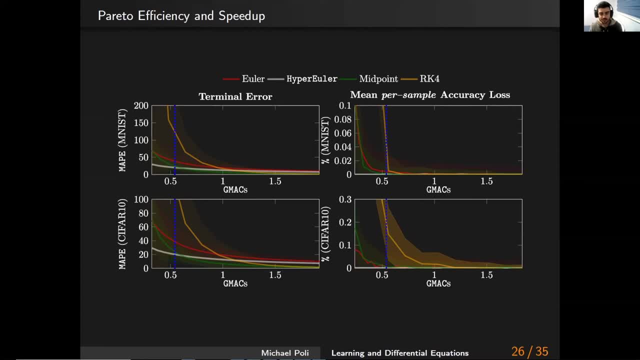 on, like deployment or or your, your needs later on, once it's trained. i like to stress, this is once it it's trained. we're looking at how you- you could use this also for for training, so there's more technicalities involved, but you like to have a discretization that preserves as much as possible. 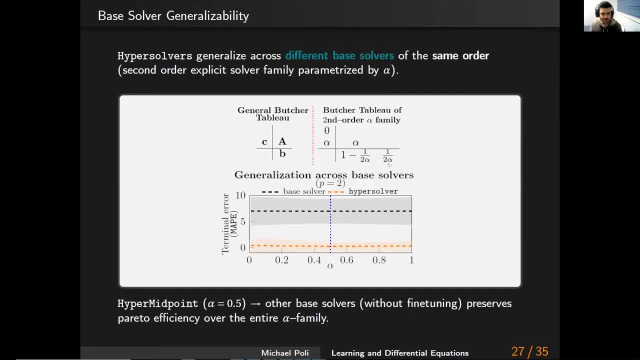 of solution accuracy and task accuracy. something also interesting, um i quickly mentioned, is that you can generalize across base solvers without fine tuning. so you, if you, if you consider a second order, second order family of software, explicit solvers, uh, it turns out there's a. there's such a thing. 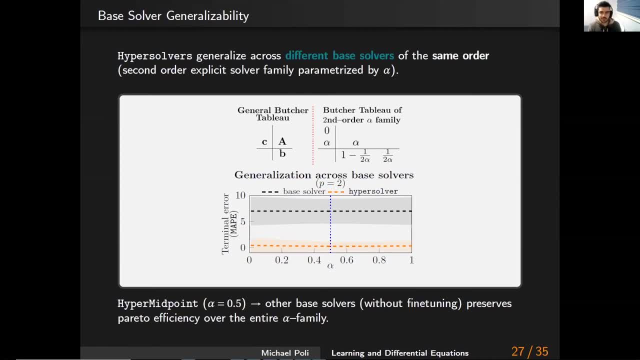 as a parametrized um family of solvers. so you can tune this scalar value to get potentially an infinite number of solvers if you, if you train your hyper solver, uh, with alpha zero point five as its, its, its base solver, and then you evaluate, without fine tuning, against the 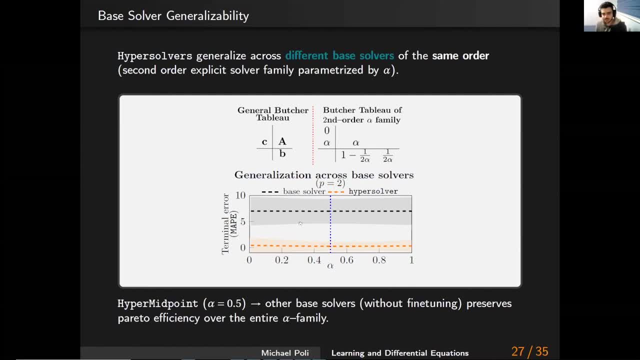 equivalent solver. you see, that doesn't really need any fine tuning to preserve the same parameter: efficiency. there's more to say that there's more results. we we hope this is just the beginning, but something that's really exciting is that we see this as as a link or as a as a similar. 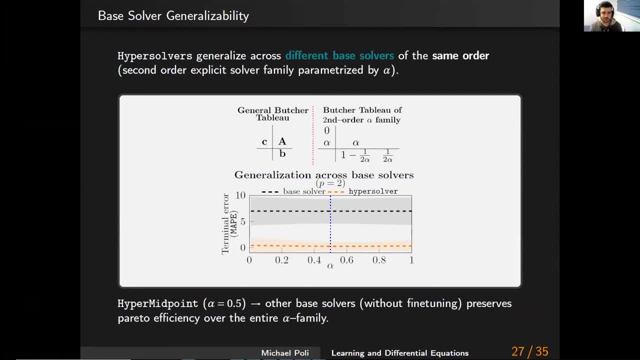 way in which nlp models- natural language processing models- have been successfully pre-trained on large corpuses of data for better performance. we see this as something similar for neural ods, in that you you might have a general hyper solver that's pre-trained on a large corpus of dynamics. 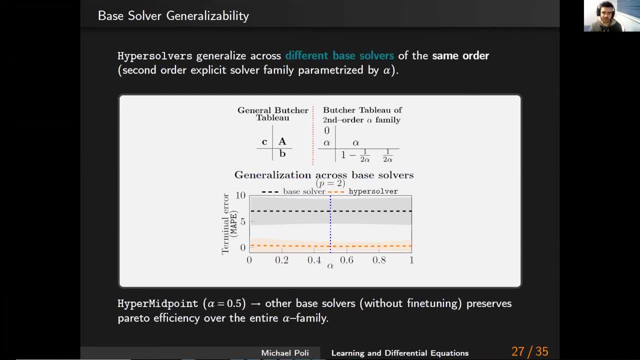 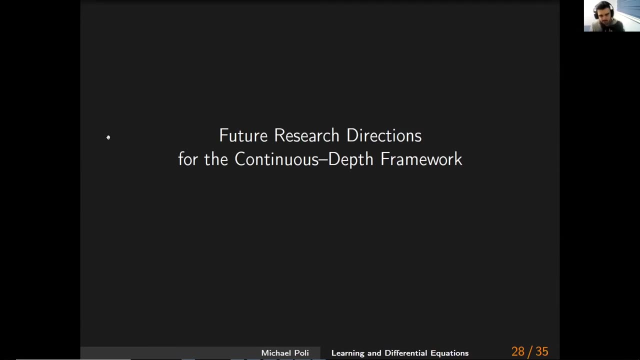 of fixed dimension, for example. and then you, you can use this to train and infer neural ds, neural sts, so sort of a pre-trained large numerical methods. not too large though, because there's uh, um, there's another head. all right, so very quickly, some, uh something to whet your appetite, if you want to go beyond neural ds. you don't think you know these. 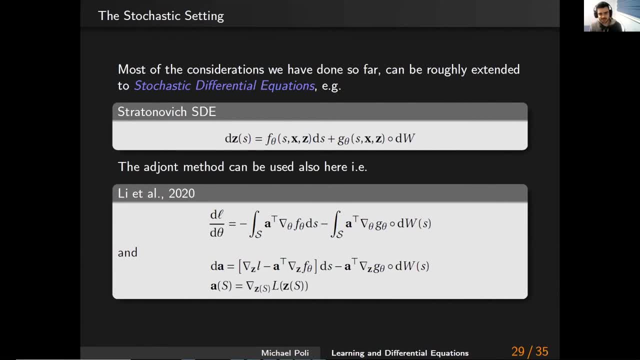 are interesting. i know many of you are uh into finance. i also have a little bit of experience in finance and this is one of the questions we get the most. um, are neural sds used in finance? can you expand your support in your sds so universities? you can already play with them in thorstein, our library, and pretty much everything. 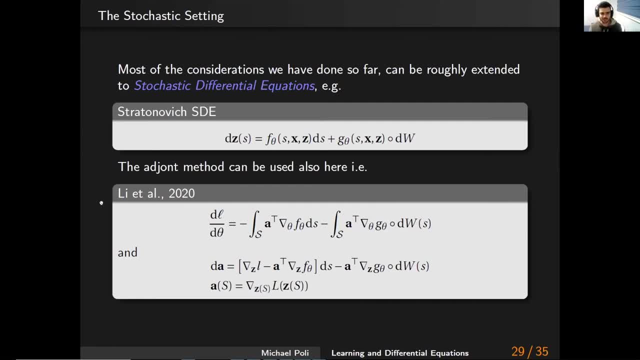 i've said so far applies to them as well. in terms of training, their joint training holds holds for them as well. pretty much the same, the same formulation: um. we have um. this is a very active field of research and we expect a fairly large impact on finance as more uh experts in. 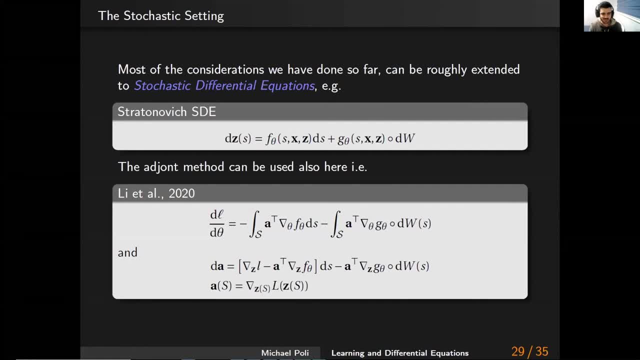 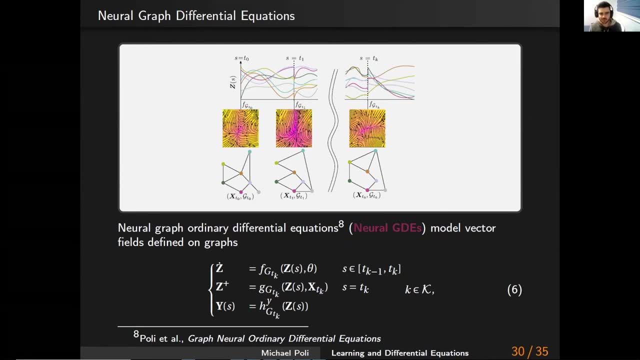 domain experts will, uh, you know, start um exploring with, with these graphs. so data as graphs is pretty much ubiquitous. you can, um, you can- have neural ds on graphs- it's called neural gds- where you have now a vector field that's on a graph so you can use your. 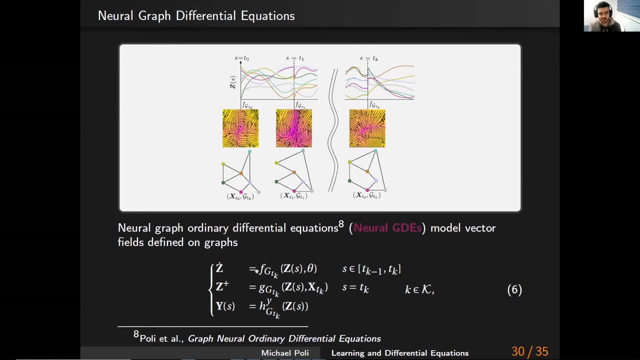 graph neural network layers as the underlying vector field where you can evolve. for example, your, your node, feature metrics z. if you, if you have a cv, you might want to have something like an rnm, like a mix of an rnm and the neural d where you evolve. 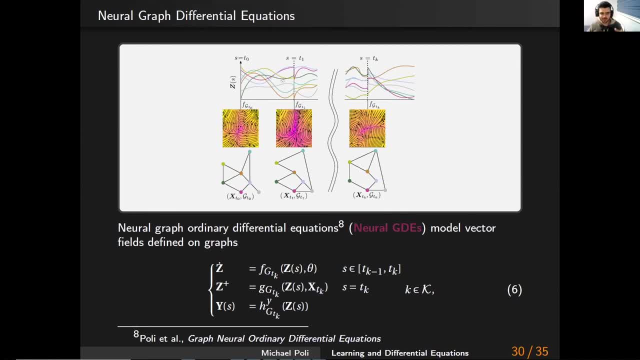 your node features in between observation times and then you incorporate with an rnm cell, the equivalent of a graph on an n cell, incorporate your graph information into a latent space and then you flow from then on. this is also a new, a new field of research that has already attempts with. 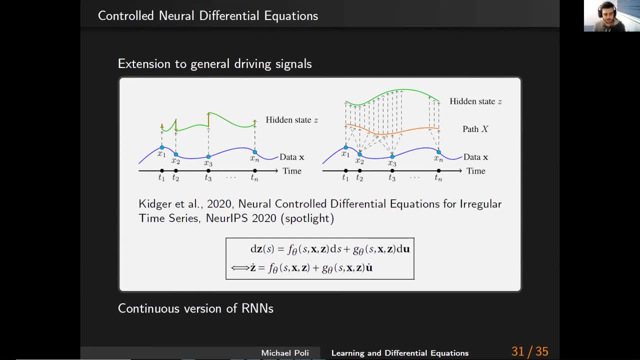 um, uh, stochastic, uh, so neural graph, stochastic, differential equations. so this is also a new field of research that has already attempts with um, stochastic neural graph, stochastic differential equations, um, if you want a true continuous version of rnns, um, you can have a full solve. so if your your data, 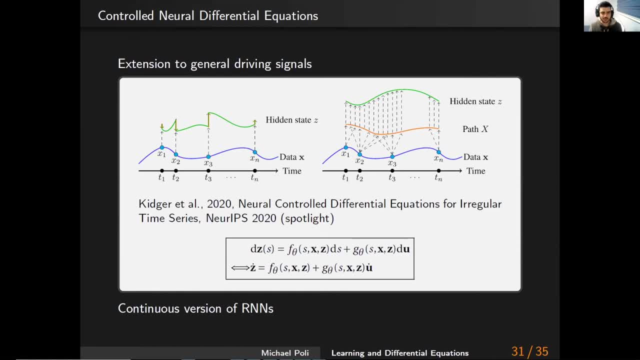 is not just an initial condition but it's a time series. for example, and you don't want to have an hybrid between uh, you can add an n cell with stm cell and then your od in between. if you want to solve everything with one od, solve. for example, you can look at control differential equations. 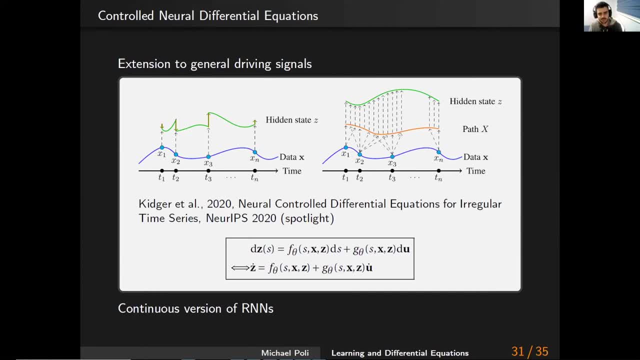 where you can, for example, you can look at control differential equations, where you can, for example, interpolate your data and you can, you can condition uh the vector field on this interpolation. you have different values here affecting the vector field. uh, this roughly the theory of control differential equations and also rough differential equations, if you're familiar. that extends to the stochastic. 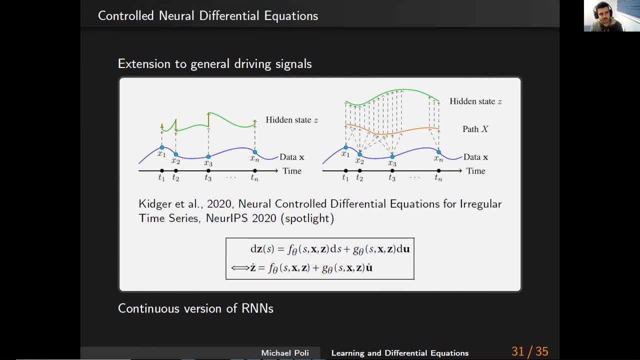 case is um really fantastic as um. it's a way to, to tie your intuitions together once you start playing with these objects. so what you have is a um, you know you, you have a, you would have an integration on on time or depth, but you also have 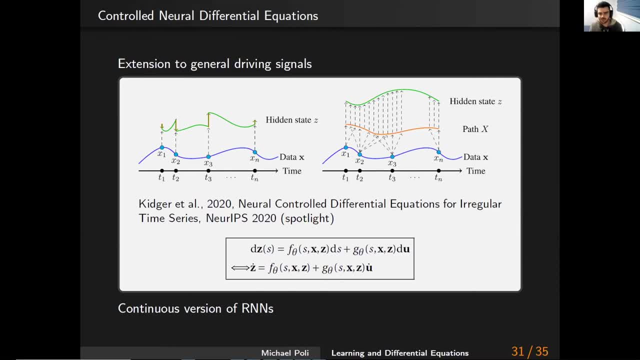 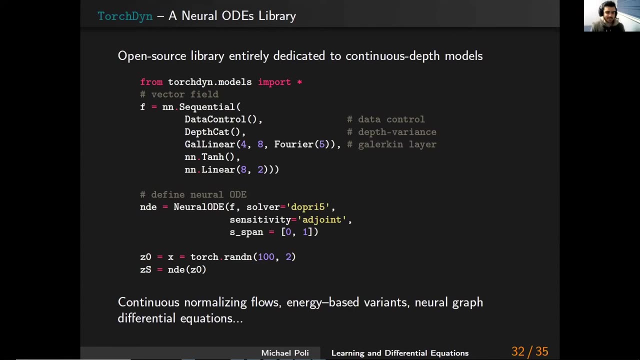 other driving signals. so for an st you you'd have your brownian motion, but here you can have other objects like an interpolation of data, but you might have a, also a stochastic driving signal. that's nothing like a brownian motion. really opens up your, your creativity, okay, so i think 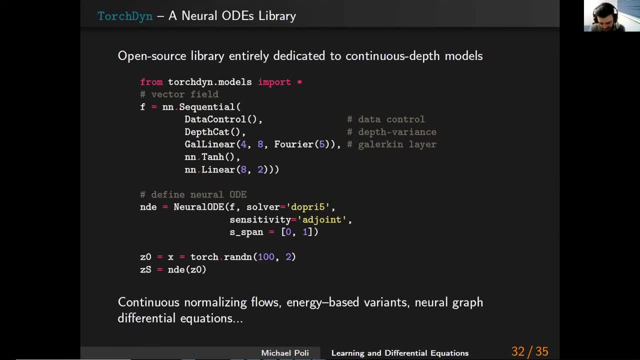 we're um reaching the end, so we'll look um. i think i'll be really quick with the code um, but i'd be happy to to answer on slack. so we have a really active sort of active slack, but i really encourage you to join. uh, we have around 40 people. 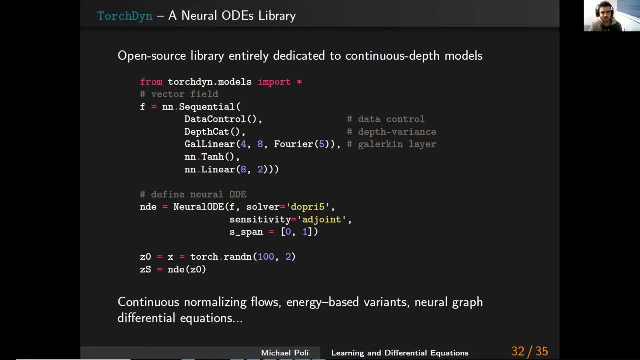 right now. a lot of researchers in in this space that you might know are present. if you have any implementation problems or any ideas, feel free to join. so this is what some of the code we'll see now looks like. these are some of the other ideas, um. um, there are some other ideas, um. 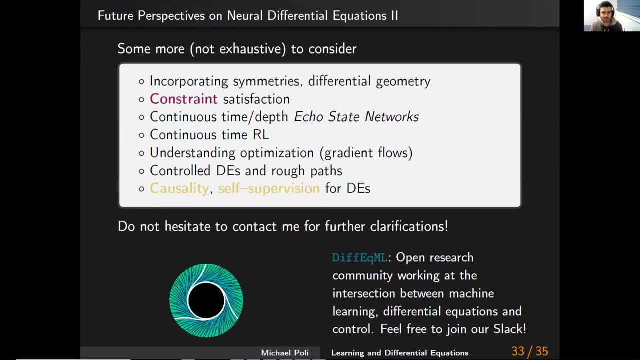 um and some of the other ideas are still working progress. there's a lot more. it's really opening up and i expect a bigger and bigger percentage of ai conferences next year to be about continuing step learning. this is our open research group. so, again, um, feel free to contact me anywhere, but also 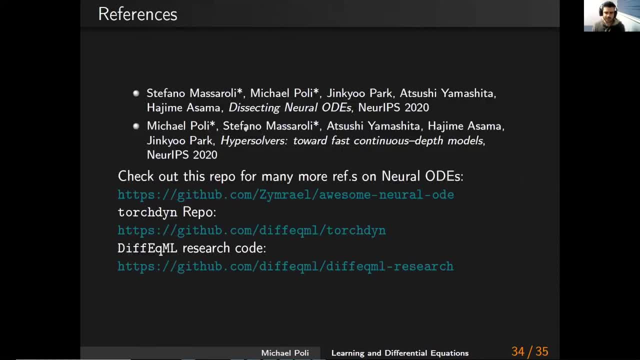 on slack. um, these are again some, some references. uh, i maintain a repo with a lot of the latest papers on your ods and your differential equations. uh, this is our link to torstein. maybe i'll share the slides later. and, uh, our hoax can, or i can, share some of these links later on. 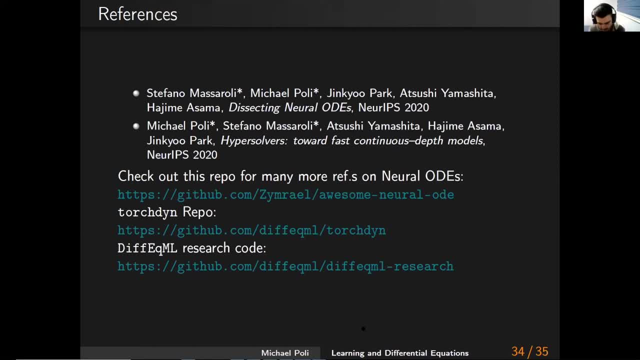 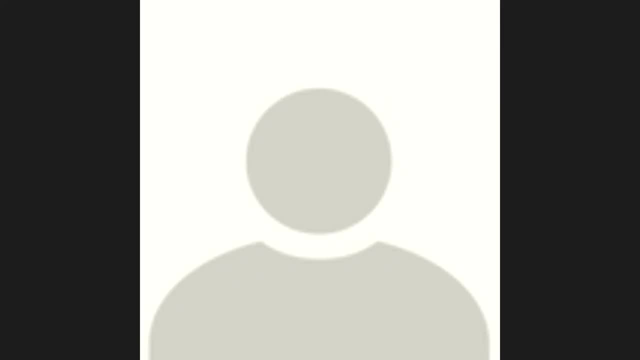 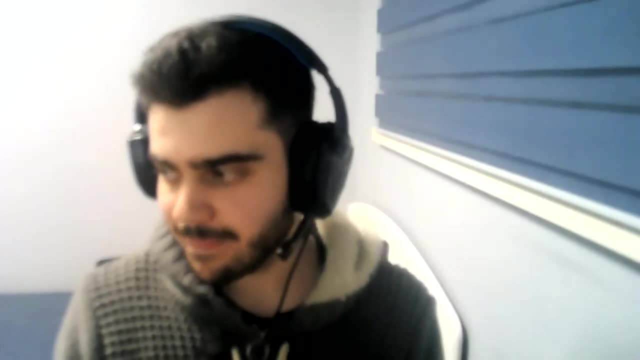 all right. so now one moment, uh, we'll take a look at the code and then we'll do some q a. okay, this is the fun part i know for many of you. i hope we can do it justice. okay, so i'll be a bit brief because i 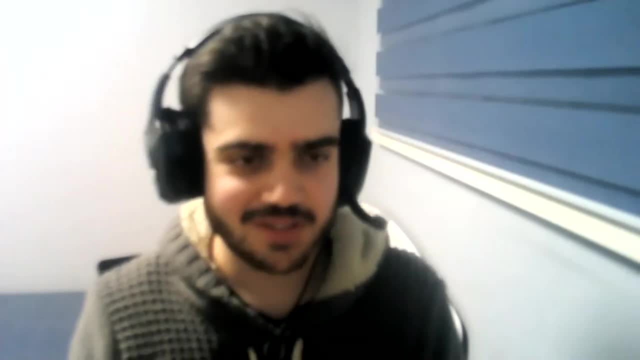 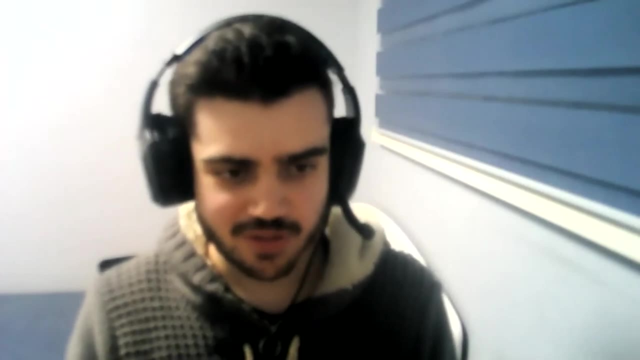 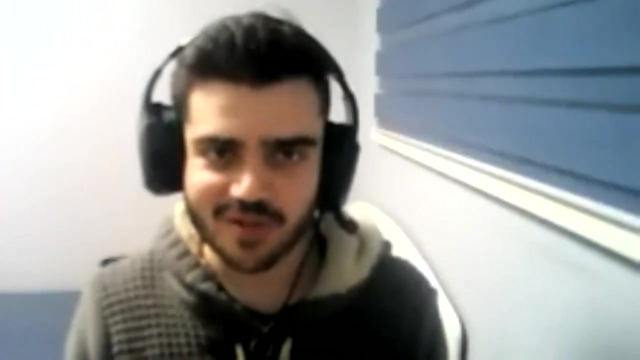 really, i really want to hear your questions and, uh, talk to you about this. um, okay, so there won't be any live coding because we don't have time. i want to show you a few things you can do. so we talked about neural d's for a while. let's see how- how it's like to train one. 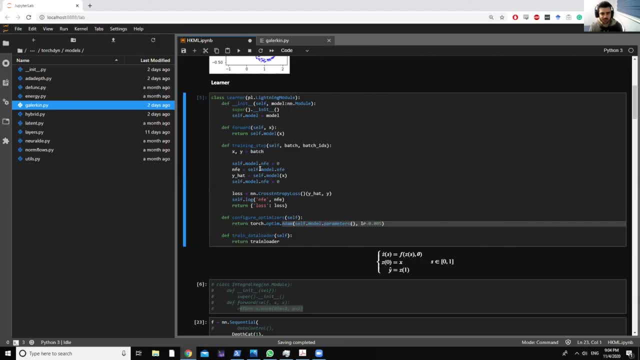 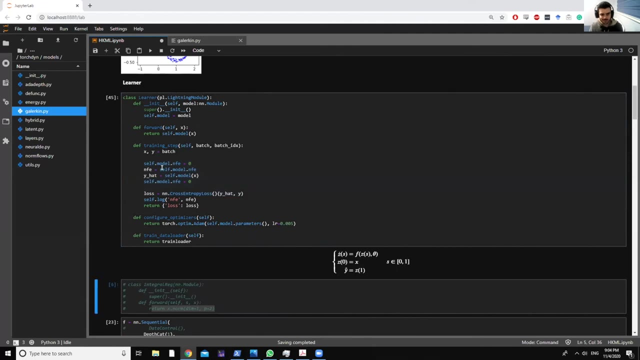 on a binary classification task. this is just a training loop. um, we're using pytorch lightning, which i i greatly um recommend. it's a way to reduce your boilerplate, but this is just a training loop. so, again, i'm assuming you're familiar with uh, pytorch, or at least tensorflow. 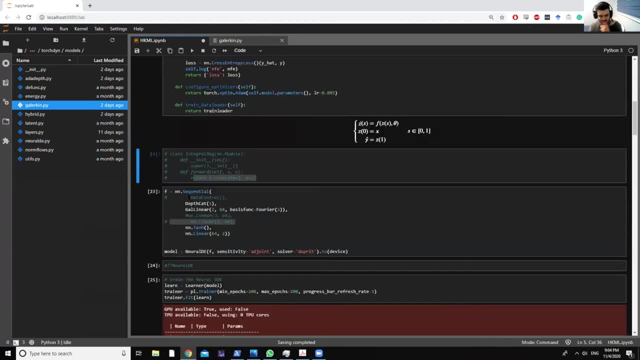 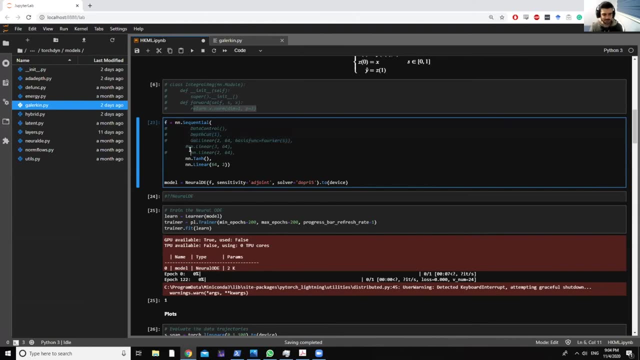 to follow, otherwise it's gonna be confusing for five minutes. i apologize. okay, let's say we have a vector field, um, that's just a very simple um. just a very simple um. nlp of this type, right, very shallow um, you can define a neural d or a neural d object and they're. 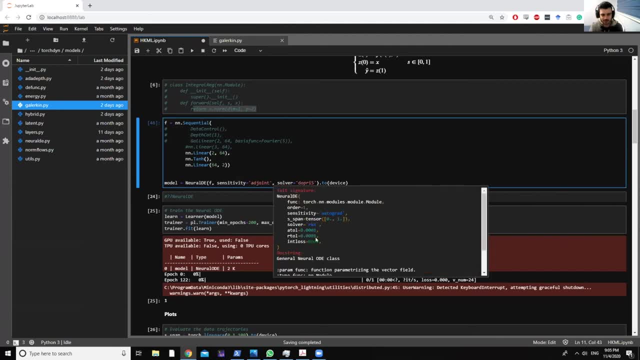 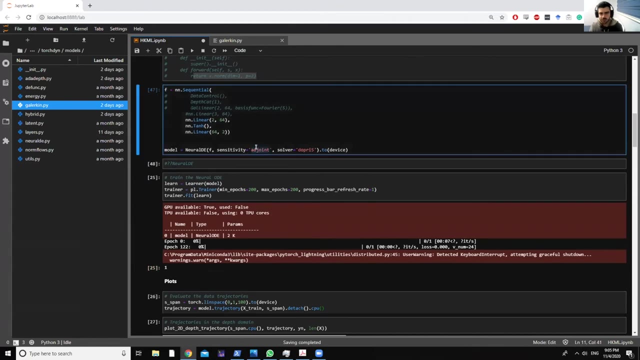 both okay, as follows: you have a bunch of options to to choose. this is one of the core classes of torstein, but we have one for sds as well, which we'll see later and there's going to be more. so what you do then you can choose between a joint and an autograd to back propagate through. 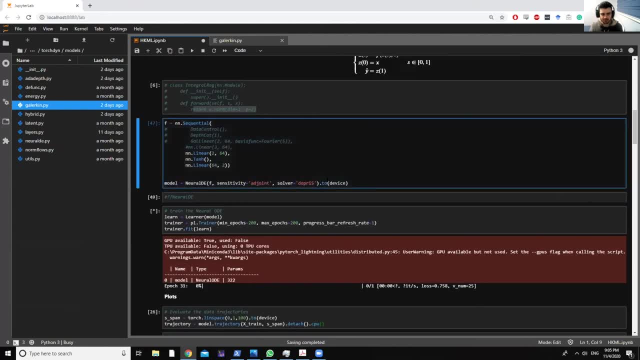 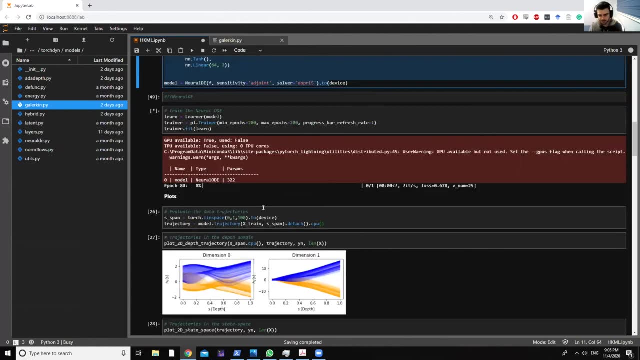 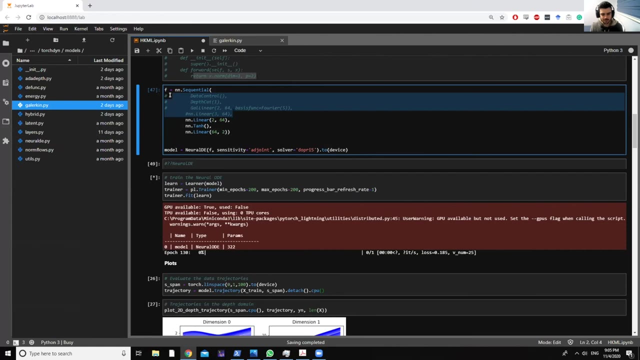 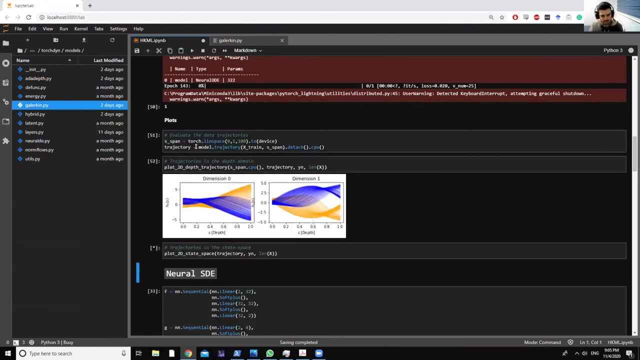 and you can. you can simply train right. there's nothing. there's nothing mystifying about this. i want to show you how the flows look, and then i also want to show you, um, the difference if we use a depth varying version, both in convergence, as well as the actual flows. okay, so with a neural d object, you can. 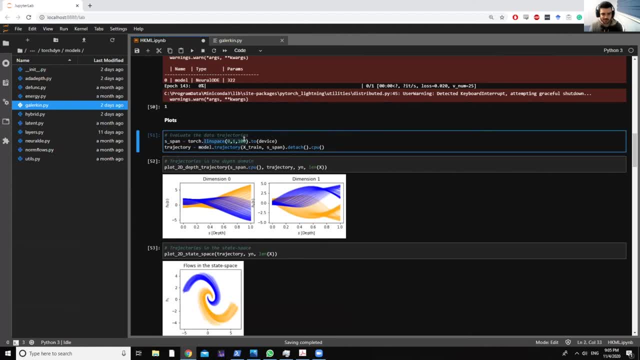 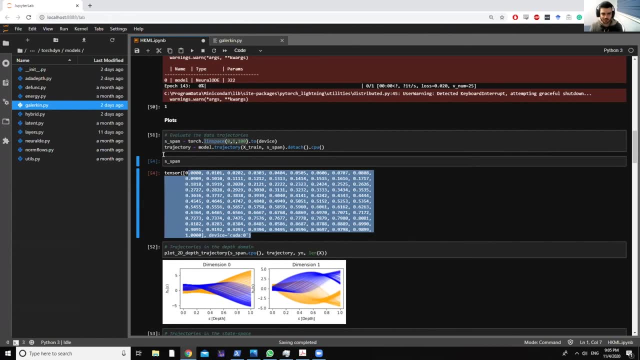 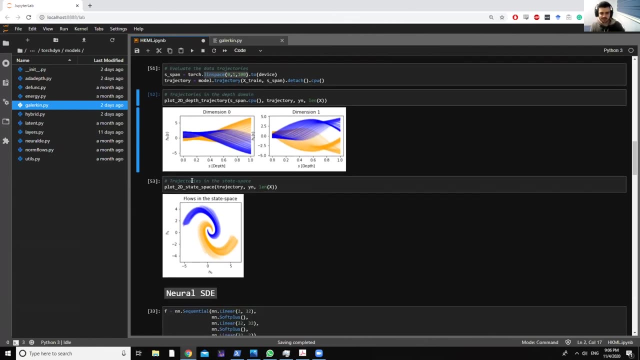 construct the flow at a certain set of points, right. so as span is simply collection of points in depth where you want to evaluate your flow, and this is what the two dimensions look, this is a two dimensional classification problem and this is what it looks like in the state space. so the two 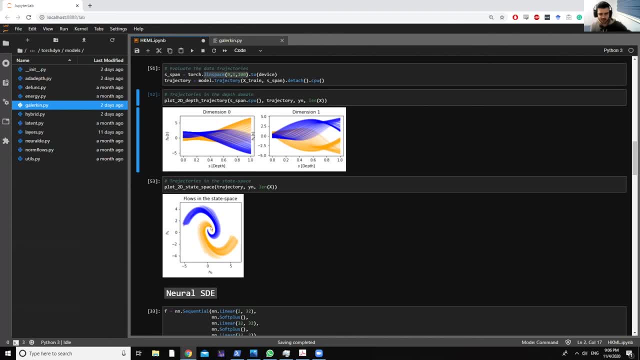 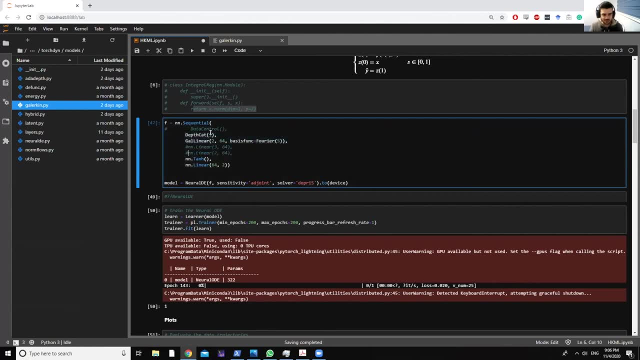 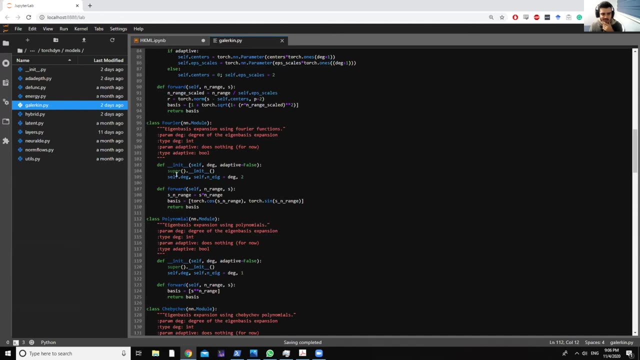 dimensions against each other, right? this is the initial condition. we're trying to pull them apart, as you saw before. now, what if you want to use depth varying parameters? well, it's really simple here. we have a variety of eigenbasis. you can choose chebyshev, polynomials, rbf, radial basis. 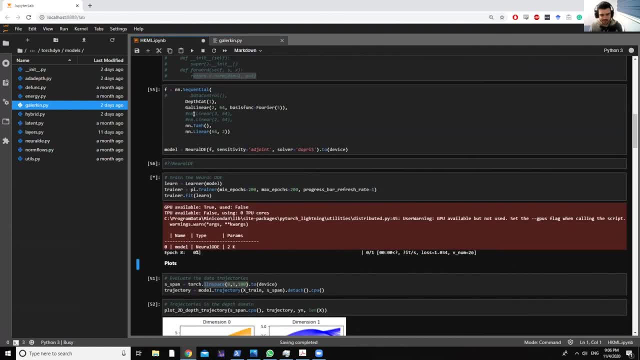 functions etc. looks exactly the same. this is also very useful, a trick where you you can include a dependency on the depth variable itself, an explicit dependency. what this will do, it will concatenate along this dimension here. so this is a nmlp, so we'll just be using linear layers, with the first dimension being a batch size. 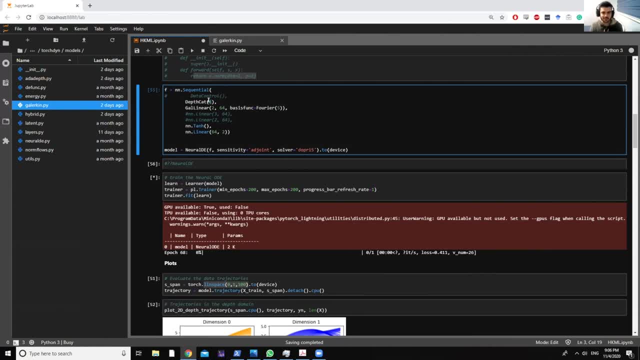 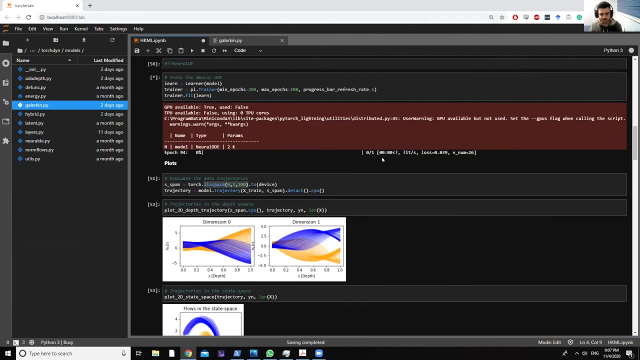 we'll be concatenating s along the, the first dimension, to, to feed it into the layers below. so if you want to use this, you can also have um. you can have an exclusive, like an only concatenation dependency on the depth variable. so you see it's. it's converging a little bit faster, although it's taking longer to evaluate. 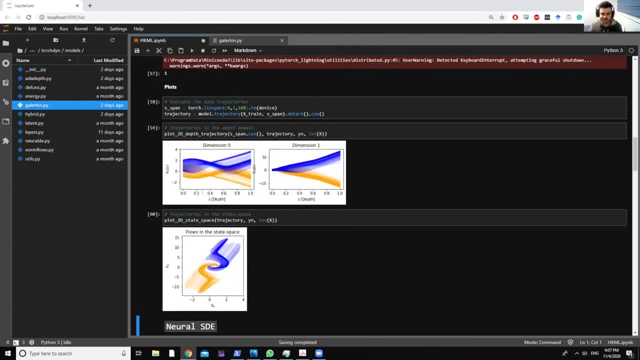 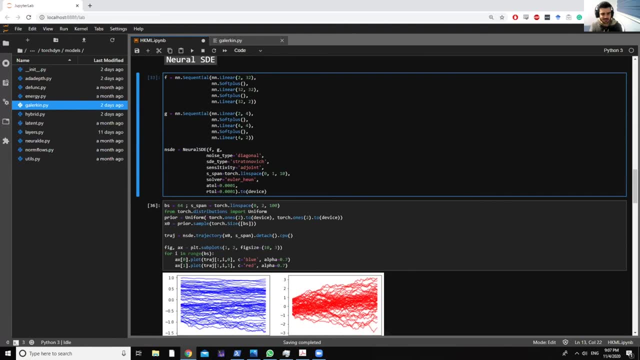 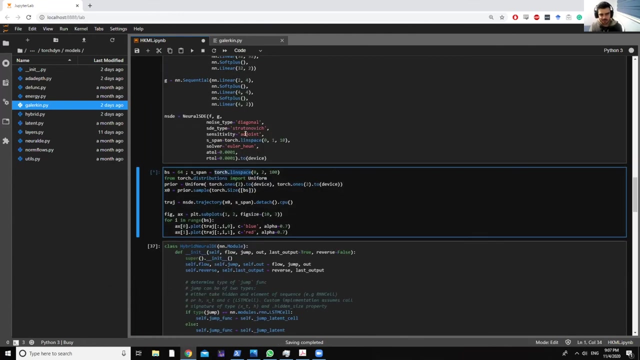 because these flows are more, a little bit more crazier, more dynamic. why, if you want to do something else, sds for the finance guys, you can specify your drift and diffusion. you can have stratanovich, eto, the noise type bunch of solvers. it's the same api, so it's kind of in space again, a joint versus autograd. 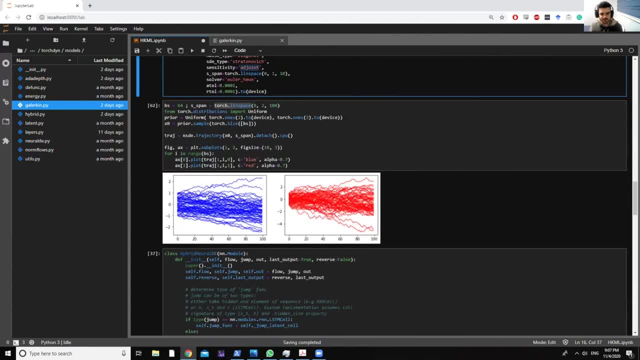 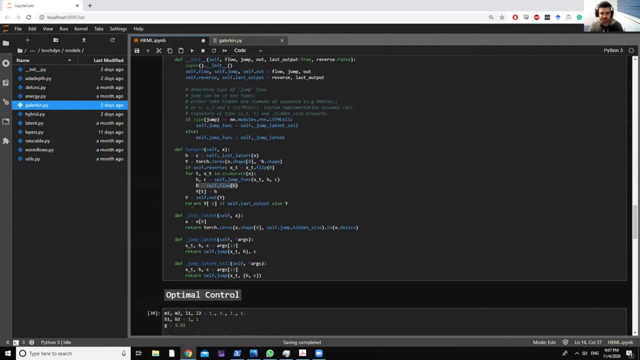 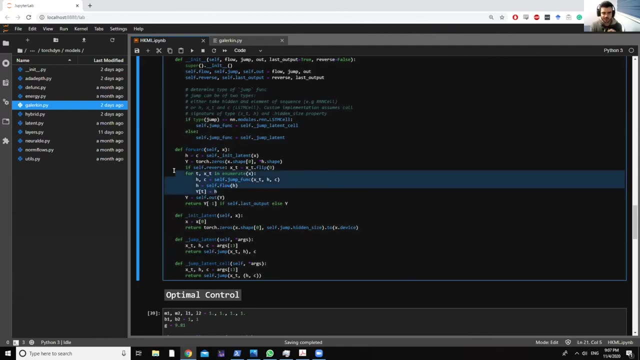 so you can. you could solve the same problem here with uh, with new sd. if you want to do stock price forecasting with this, you might have to put it into an hybrid module where you're doing jumps, as we discussed with neural graph differential equations. you will have a for loop. as you step through your time series you will have a jump like an rnm. 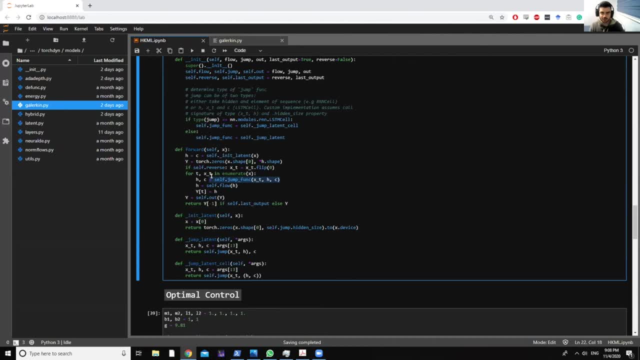 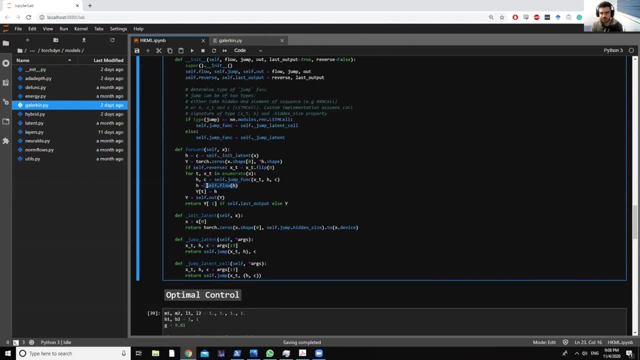 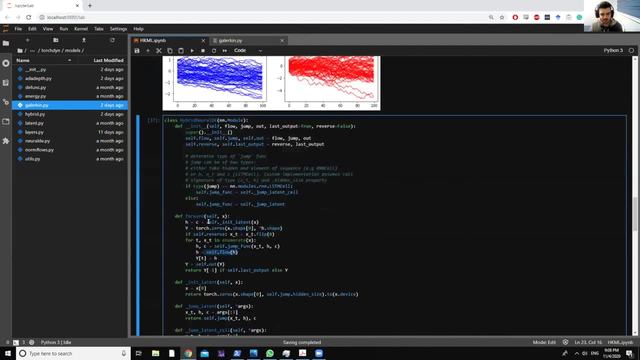 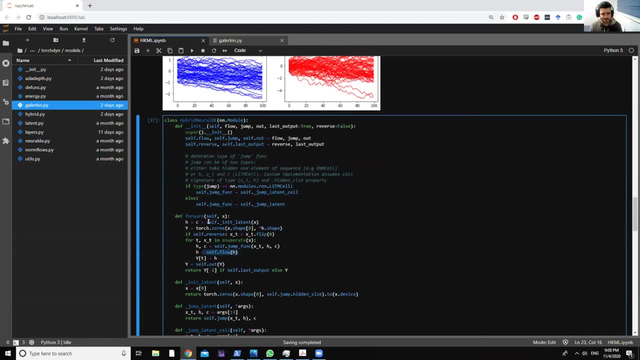 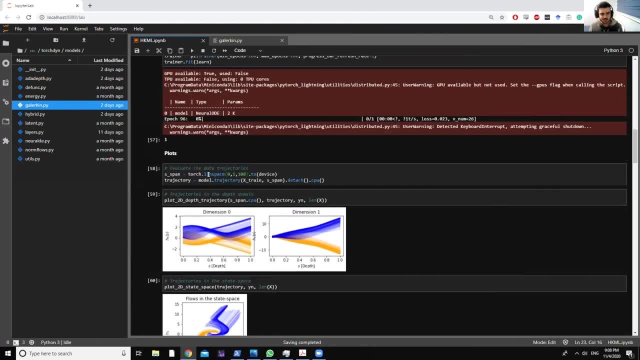 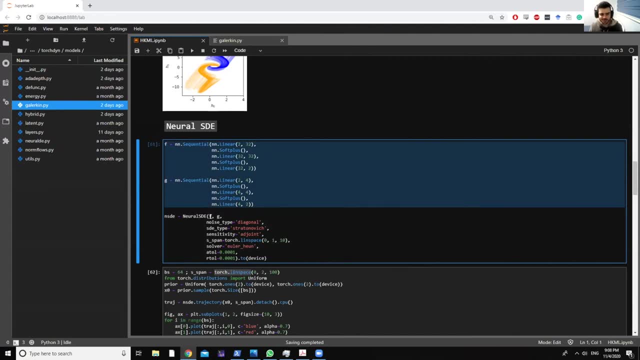 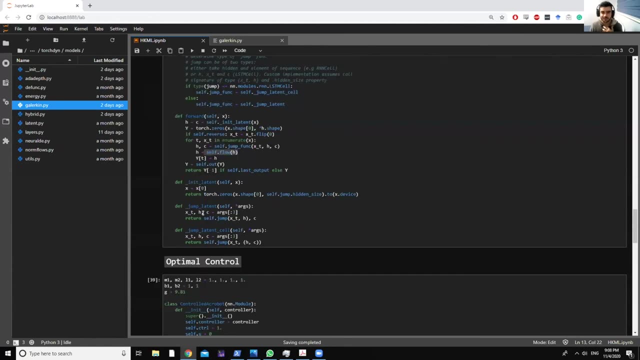 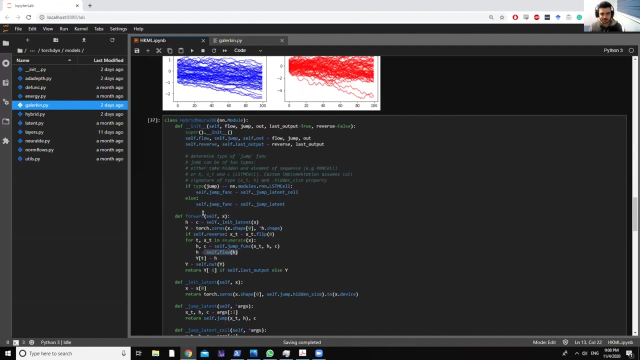 you need to. that is about the question. or faster, no, no, my. so here I know some others. I want to learn. I want to do control. You can do it, no problem. So you want to do control of an acrobat double pendulum. 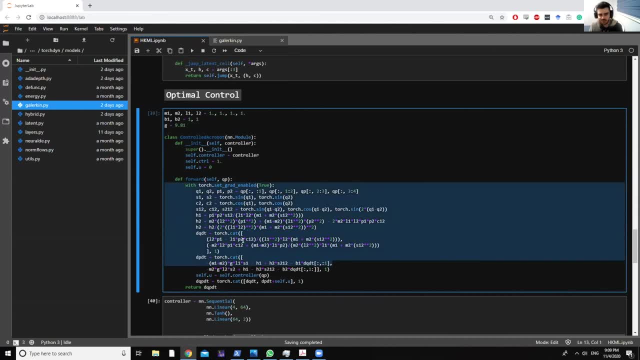 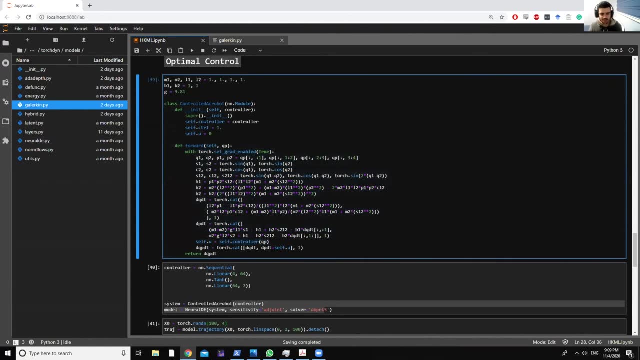 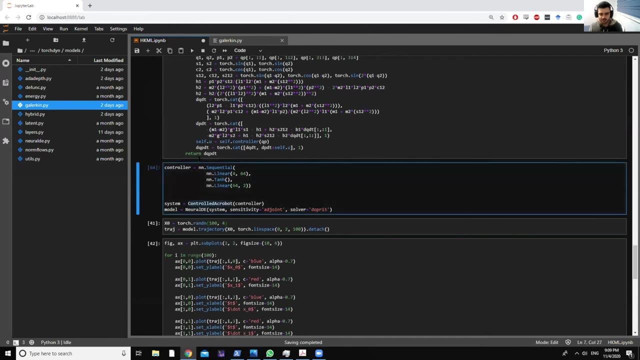 You have your dynamics equations. They're not very pretty, but you have them. You can say: I know my control enters the system this way. I want my controller to be parametrized by neural network like this: right, Then you create your. this is your ODE system. 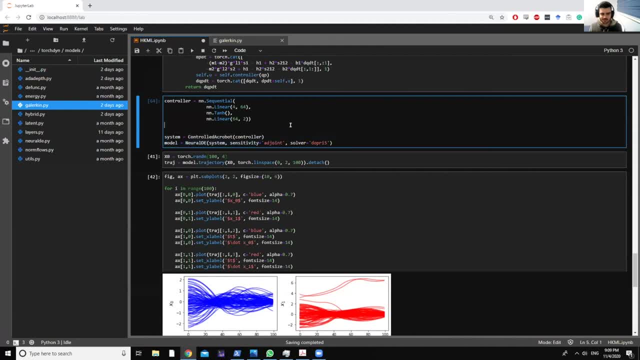 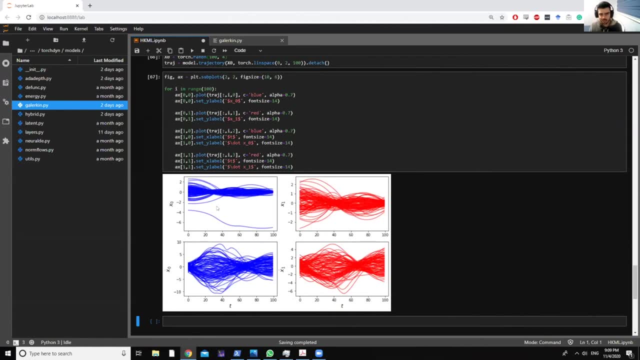 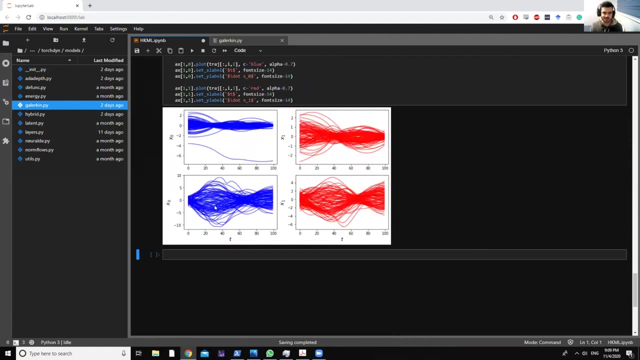 This is your vector field that goes inside the neural ODE. Then you have access to the same API, right. So you're solving the system, the control system in batch and GPU, and you can solve an optimal control problem. You can say: I want to stabilize the system. 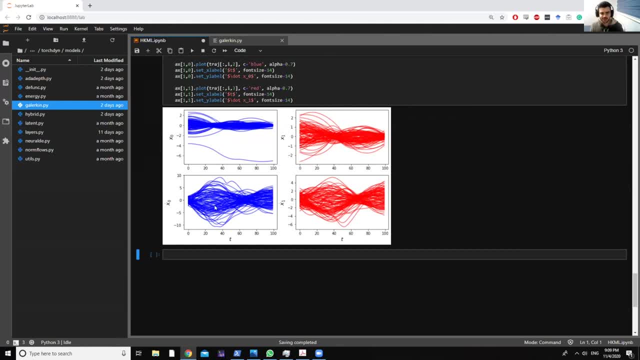 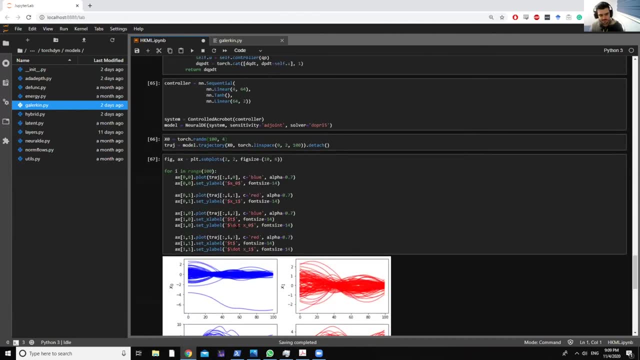 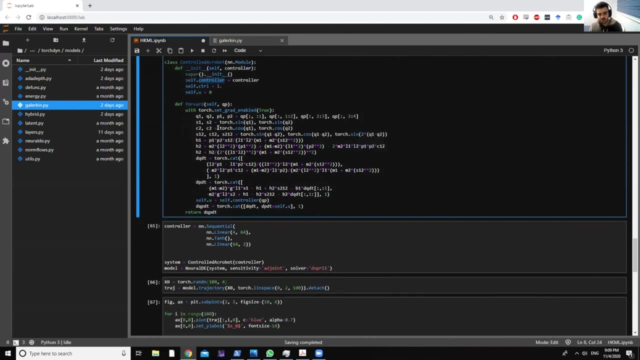 on this point you have your cost function. That's maybe the norm of the state and the endpoint of the solution of the ODE. Then you can iterate and optimize the parameters of the controller right, So you can do model-based control. 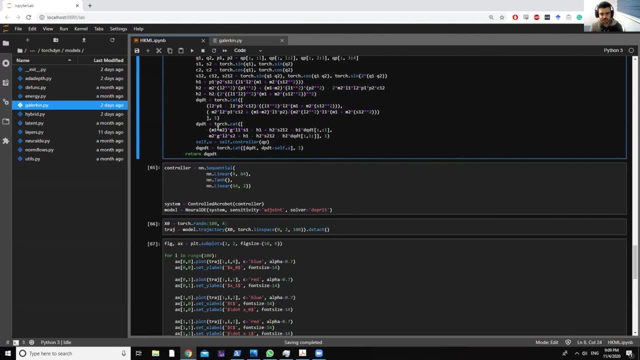 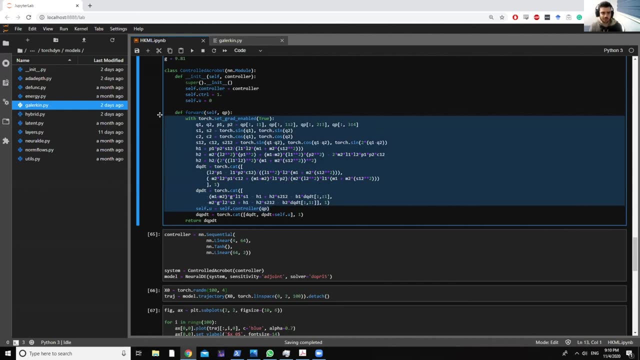 or you can go beyond. you can do model-free control. So you know you're controlling this type of system. You don't know the dynamics equations but you know, for example, maybe it's a conservative system. You know it's a mechanical system. 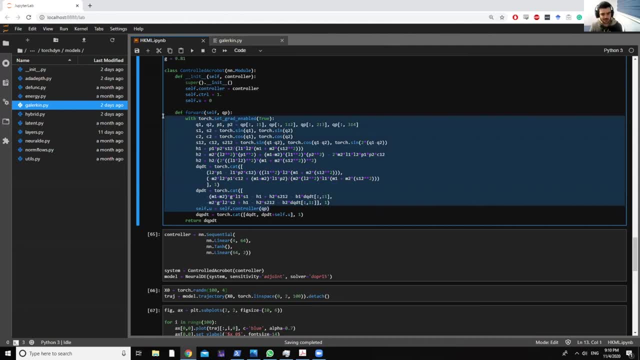 You can put your knowledge here. You can have maybe a Newtonian neural network, specific type of neural network that preserves energy. You can have a second-order type of dynamic And that's all model-free in the sense that there's a neural network that's approximating everything.